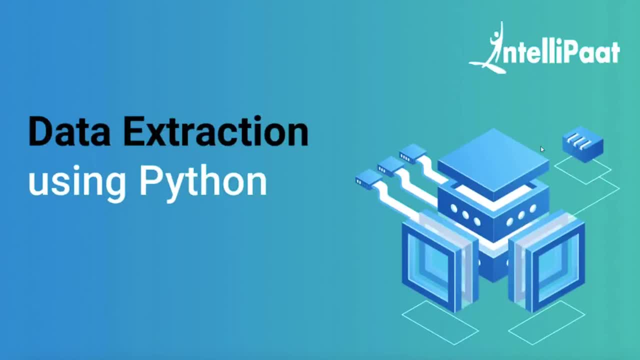 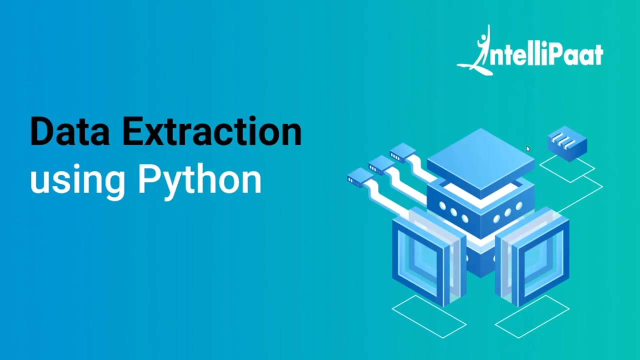 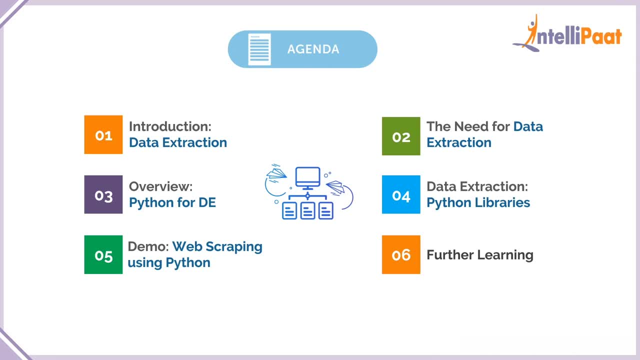 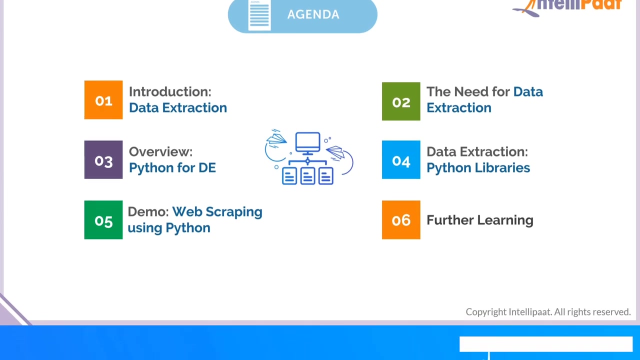 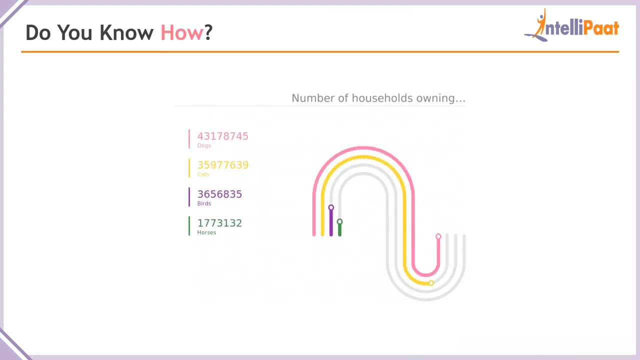 To start out with, we'll take a quick introduction to data extraction. After that, we can understand the need for data extraction and get an overview of how we can go on to use Python To achieve data extraction. After that, we'll check out some of the very good Python libraries that there are available for data extraction And at the end of it, we'll check out a demo where we're doing a quick web scraping project using Python. And, last but not the least, I'll be guiding you on the quickest way you can become experts in Python. So well, before we begin with the first item of the agenda, I want to ask you guys if you know how this works. Consider this graph on your screen right now, So you'll see a couple of statistics here. 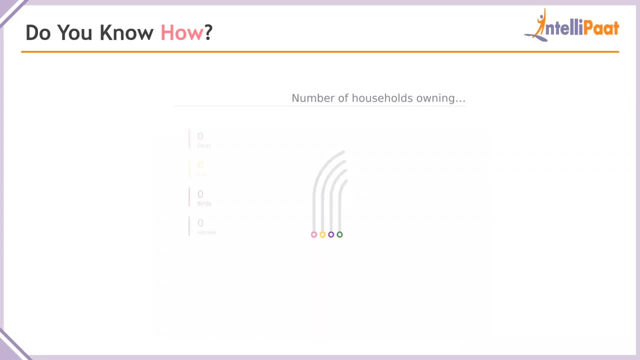 So this is basically telling you the number of dogs, cats, birds or horses, or any pets in general, that a household might own. Well, how was this statistic derived? You know you cannot go on to probably survey every single household on the face of planet Earth to probably get this information right. So this information will be extracted from a place, from multiple places in fact, where there is some detail given about if people are owning dogs, cats, birds or horses, for example. So this, what we're going to do, is we're going to take a look at the number of dogs, cats, birds or horses that a household might own. 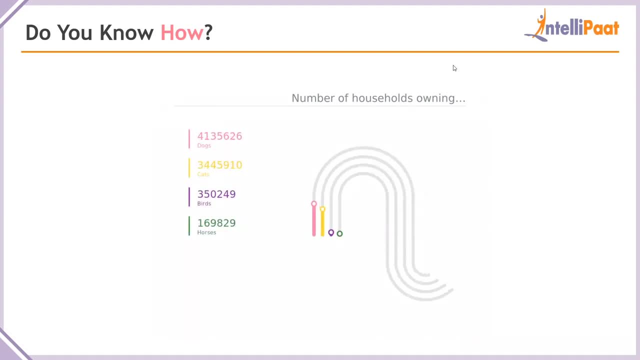 So what you see on your screen- the very good looking animation, of course, but more importantly, the detail that you see in the screen with respect to the numbers- is the exact result you know one can obtain of data extraction. Of course, there are millions of you know other results and other staggering numbers, or you know achievements that you can go on to have when you're making use of data extraction, But I thought this was one very nice case of what happens and what you can actually obtain by making use of data extraction. 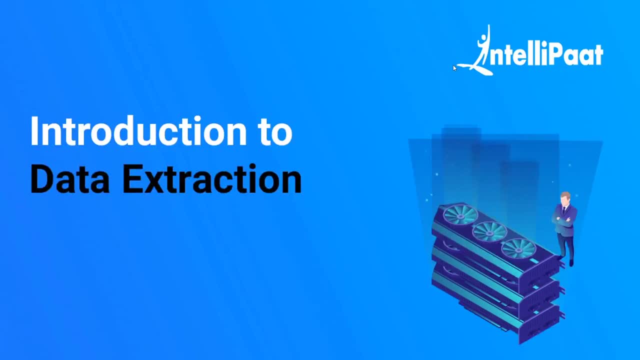 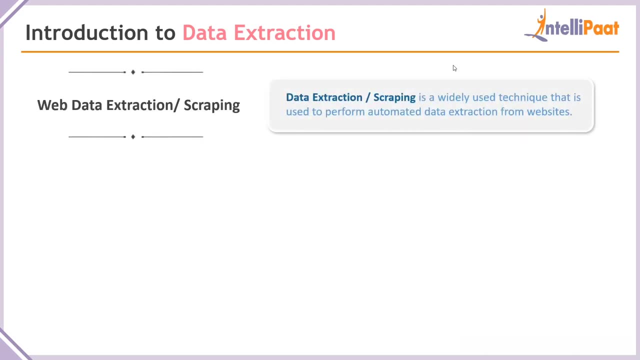 All right, All right. This brings us to a quick introduction to data extraction. So when we talk about data extraction, what is it exactly that we're going to discuss? The first thing you need to understand about data extraction, as the name suggests, is basically that it is a technique which will go on to you know. pull data from places such as websites, social media sites or whatever it is in general, And this information can be used by you and can be leveraged in such a way that you know you can go on to probably use this information. 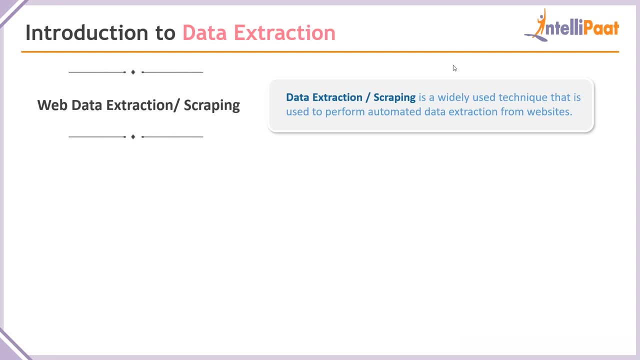 Effectively. See, for example, there are multiple things when you can consider some simple entity such as a tweet on Twitter. So people go on to you know, post things of whatever comes to their mind on Twitter, Right. So there's something called a sentiment analysis which has been coping up and which has been upcoming for the last couple of years, basically. So, when you think about Twitter sentiment analysis, you can understand if people are happy about something, if they're sad about something, or if their viewpoint is even neutral. 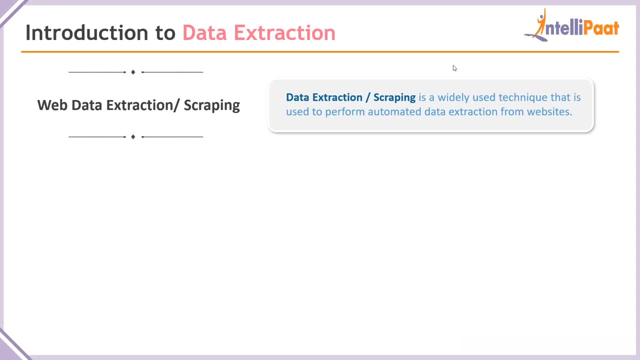 So I mean, who knew a couple of years ago That you know your post on Twitter will actually help people analyze something? So why would somebody even want to analyze something on Twitter, You might be asking. Well, you know, basically, at the end of the day, you're converting this raw data, which basically is the Twitter responses in our case, into information. 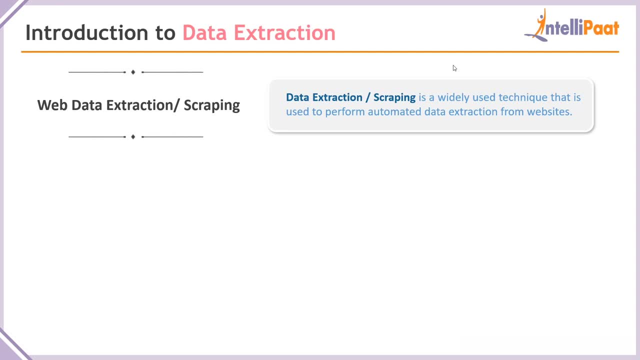 So you might be wondering if your brand is performing very well, if your product is selling well, and how happy are people when they're dealing with your businesses, and much more. So I just gave you an example which came on the top of my head right now. 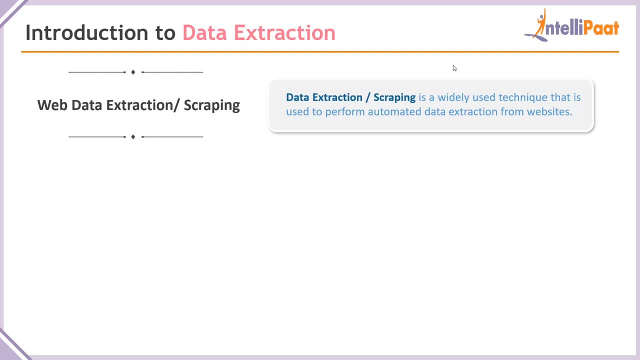 But again, I can give you a million examples, So how and where data extraction is being used very effectively. and, in fact, make sure you stick to the end, because in our demo we're going to be considering something from the present situation right now. 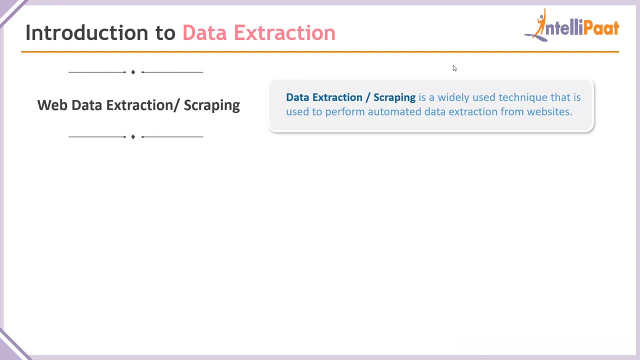 And it's going to be really nice to understand the real time use and help of data extraction techniques as well. So, again, coming back to the definition, basically what we're talking about is a technique, is a methodology which will help us, you know, gather the data, and it does it in an automatic way so that we don't have to manually gather the data. 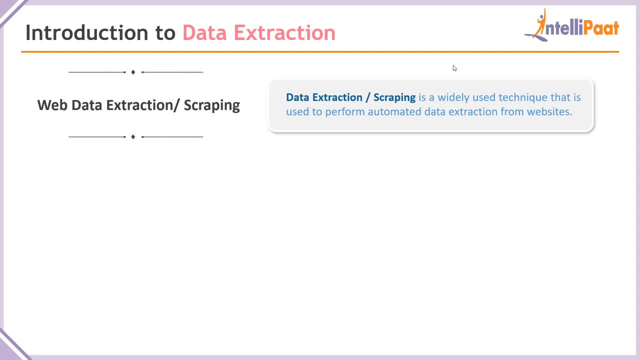 So that's what we're talking about. So this part where it's automated is all about what we're going to discuss, because at the end of the day, if it's going to be a manual task, I mean you wouldn't need a procedure to do that. 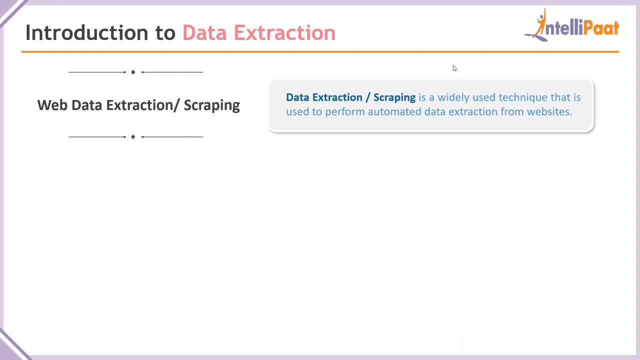 You wouldn't need a technique to do that, Right? So all you have to do is see something from a website and start typing it out, probably. So this automation part plays a huge role. So when we're talking about extracting data from websites, when we're talking about extracting data from anywhere, you need to understand that there's two types of data present in today's world. 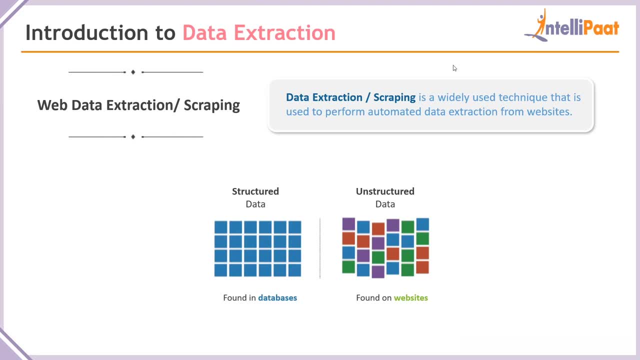 One is structured data and the second one is unstructured data. If you're talking about structured data, you know structured data will have something to adhere to, It'll have some rule, you know, it'll have some policies or it'll have basically a guiding principle behind it. 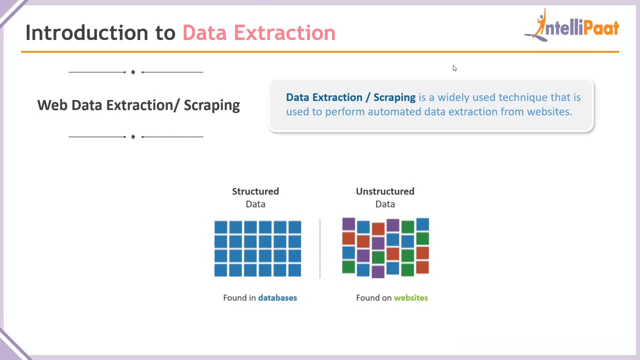 For example, when you look at the data present in databases, it'll either be of the same type or it'll adhere to all the rules of the data that is present in the database, probably. Or when you're thinking even of structured data in general, it can be just a very good, you know very well organized calendar or a timetable based database. 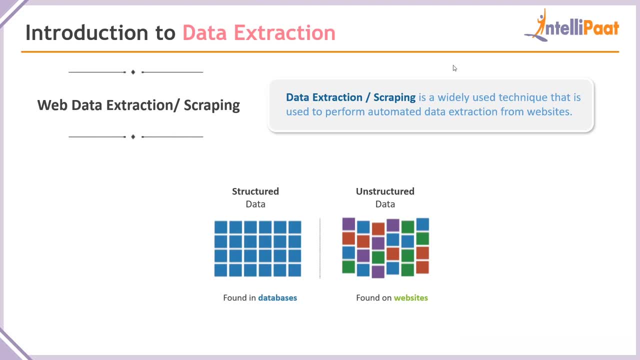 Or a timetable, basically in your calendars. So you know something from that simple entity to all the way to, for example, images. it can be audio, it can be video, data, and you know it can be anything- text as well. 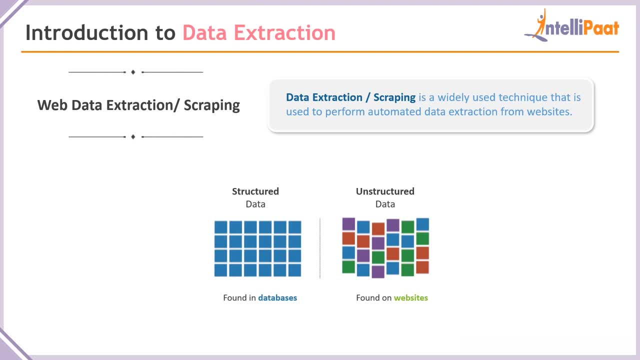 So when you're mixing up all of these concepts, your data becomes unstructured. There is no one set governing policy over the data which says: yes, you know, I can use this one rule to basically assess and control all the data. So this is a very important difference that one must understand when you're working with software. 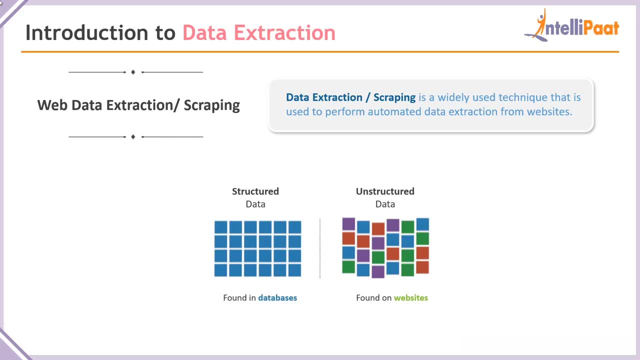 When you're working with structured data and when you're analyzing unstructured data as well. So I hope I was clear in helping you understand structured and unstructured data. Anyway, on that note, guys, let's- as always, let's- keep the session very interactive. 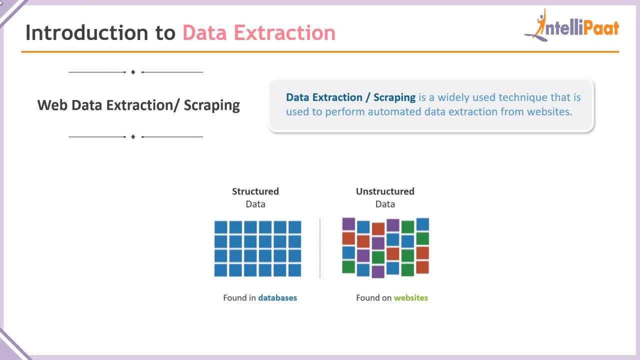 Make sure you head to the comment section and leave us all your comments. So we have our team members waiting for you guys to hit the comment section and they'll help you out as soon as they can. So make sure you hit that comment section and leave us with any questions, you have suggestions or anything you'd want from this session as well. 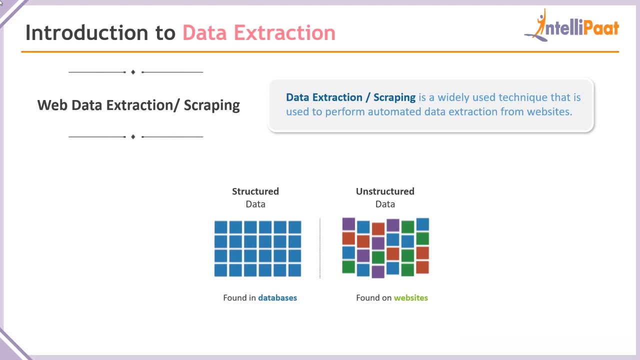 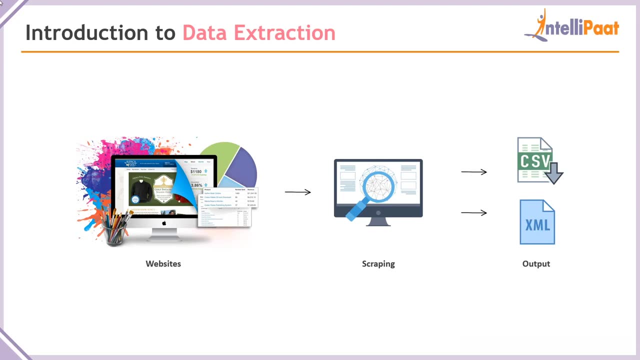 So let's keep it interactive. Head to the comment section. All right, guys? So on that note, we need to check. one more important thing is how one can go on to do this. There is one term when it comes to data extraction, especially from websites. 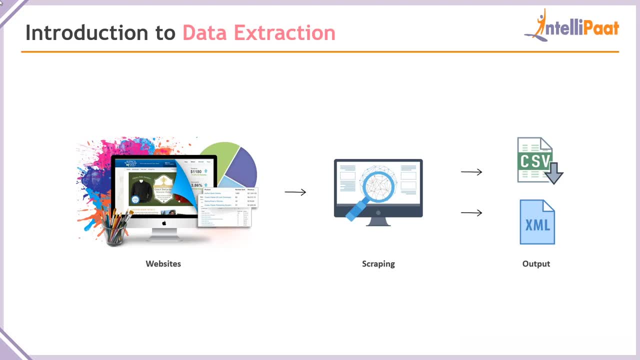 The term is scraping, See so when you go on to check any website, for that matter. Right. So all these websites, they contain images, They contain text of some sort, or they might contain, if it's a, if it's a website such as Amazon. 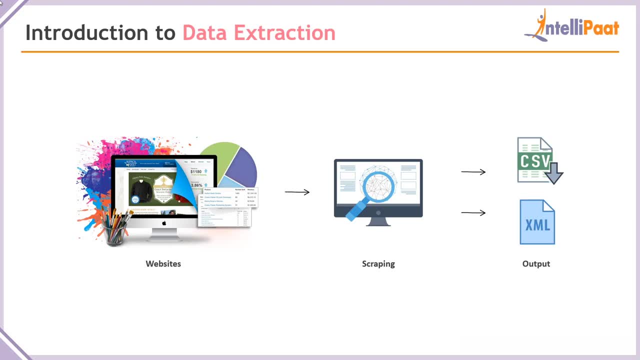 For example, any e-commerce site. you'll have products, you'll have pricing, You know you'll have situations where the product is deliverable to one place and not the other, for example, as well. So when you're working with all of these concepts, there are a million ways and there are a ton of data that you can actually gather from these websites. 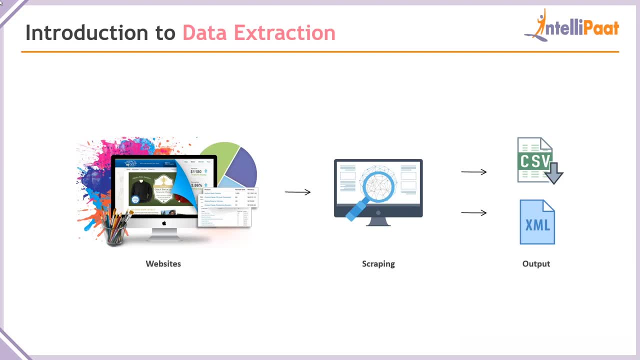 So, basically, what one can do is: you know, if you guys are into sports, you will know that the players for the teams are usually auctioned off when you're working with Premier Leagues. So when you're talking about all these Premier Leagues, 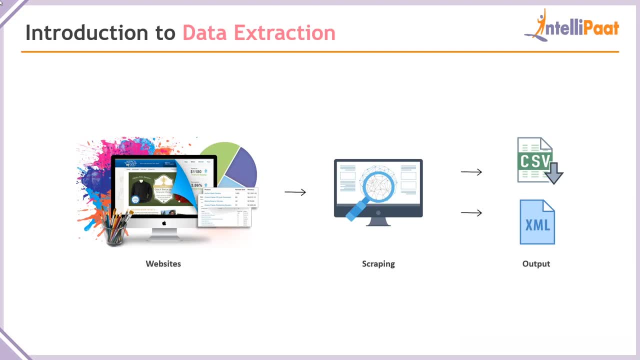 What usually happens is each player has a value and their bid on and their one. So you know you can actually go on to websites to find what the what the price of the player was when they were bought into the league. And you know you can create a very nice looking Excel sheet and you can organize to see see what player was worth what. 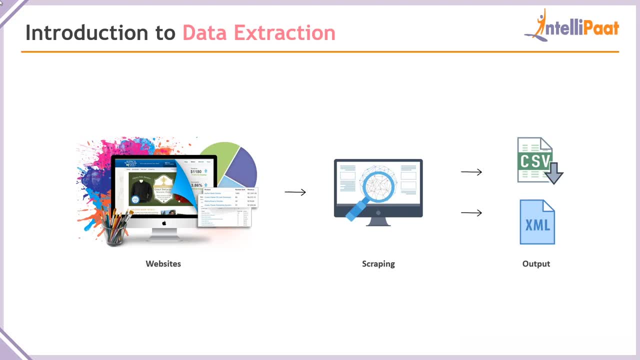 And eventually at the end of the Premier League they usually put out tables and charts with the number of goals. So you know, you can create this very fun project where you're trying to find out the return on investment as well. So again, just another example here. 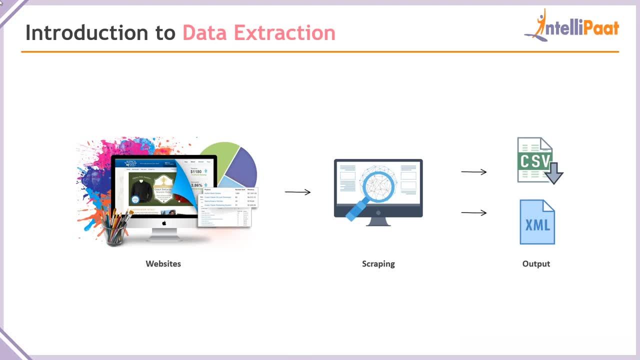 But then, to give you another example, you know you can go on to e-commerce sites like Amazon again, Flipkart. There are many other places that you can find out all the prices that each of these guys are offering for the same product. 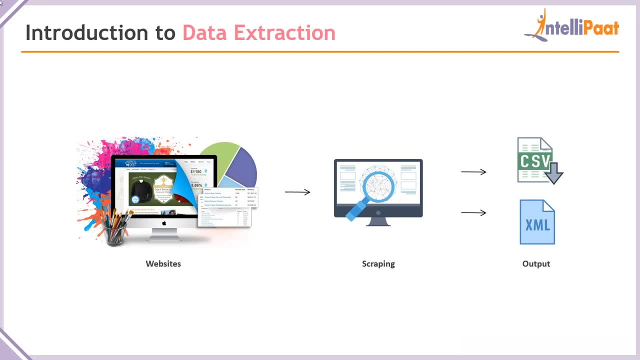 And you can find out who is providing it for cheaper. Is it Amazon, Is it Flipkart or any other case, for that example, as well. So all this information is gathered in the websites, and we use a term called as scraping to basically pull all of these information out. 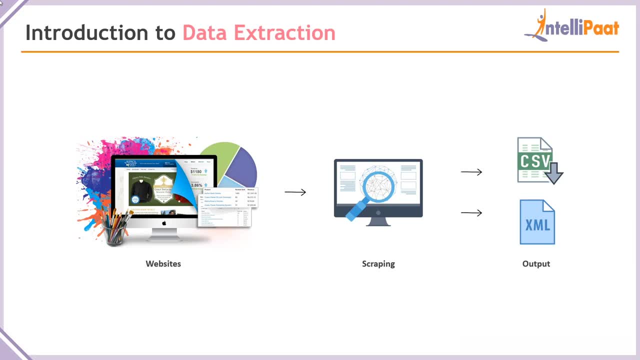 Scraping. Scraping literally means hunting for the information that you need, filtering for the information you need and basically bringing it on to your machine, or basically to bring it on to your native base, where you know you'll be converting it into files that you can use. 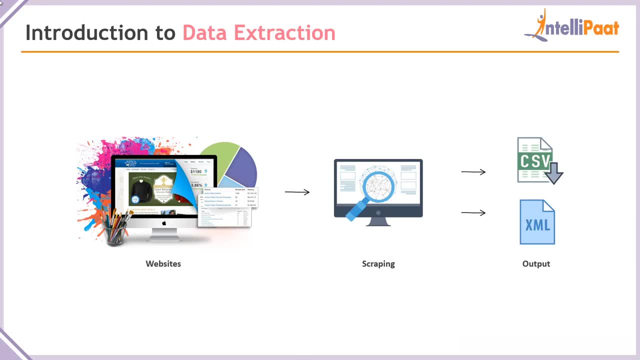 So CSV is a very structured form of storing the data. For example, let's go back to the e-commerce example. we went So you can have name of the product, the vendor, vendor one and vendor two, for example, Flipkart or Amazon. 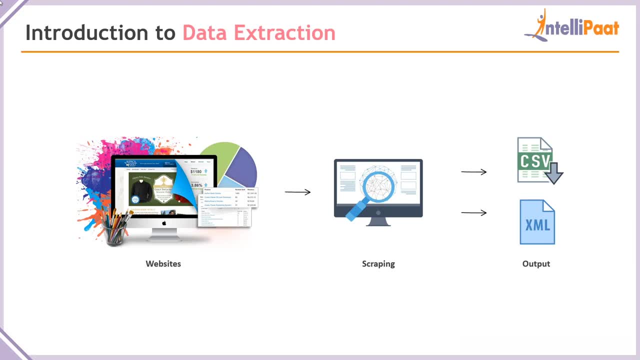 And you can get the price of both of them. You can compare and check who's giving it for a better price and what not. So this forms the basic outlay of how one can go on to, you know, perform data extraction. Data is present in the websites. 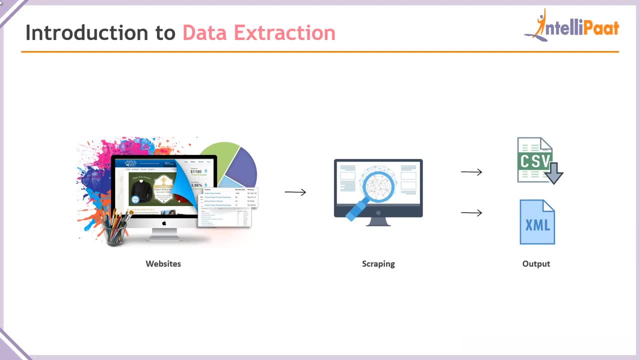 We'll be cleaning the data and pulling whatever data we require And after that we'll see if there is any processing to be needed. And if processing is needed, it is done And at the end of it we will save all of these files in a format which is basically structured and which we can use further down the line. 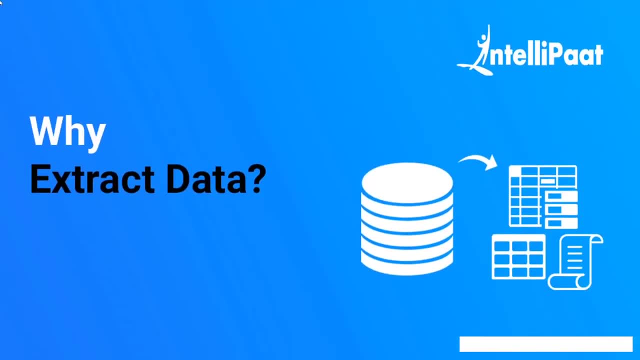 Alright. So on that note, you know you need to understand why we need to perform data extraction. Guys, again, if you know why data extraction is important in today's world, head to the comments and let me know. So, coming to the answer to why one should scrape data, 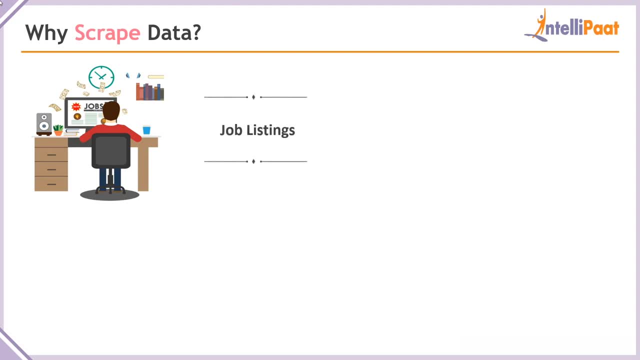 Here is a very good first example for you, When you go on to the top job hunting sites, be it Nokricom, be it Indeed, or be it LinkedIn jobs or whatever You know. So in this situation, when you have to find out, 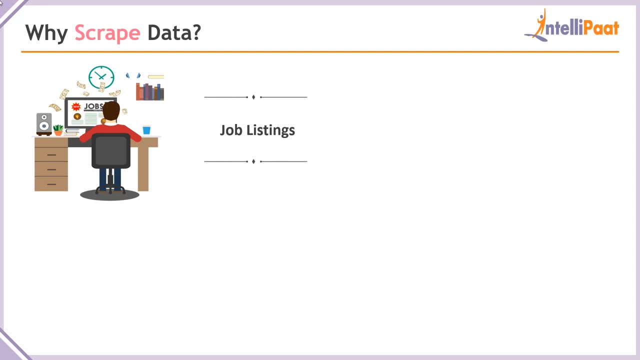 What about all of the top jobs that are present around the world? Well, it would be really nice to have all these jobs that you're looking for at one particular website, Right? So consider the situation where, let's say, you know you want to become an artificial intelligence developer. 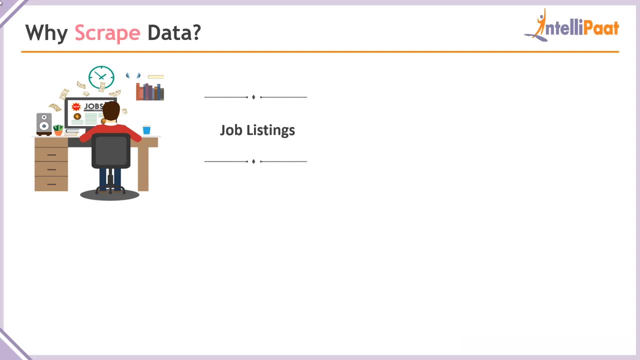 Artificial intelligence is on the rise in today's world, as you might know, and you're looking for a job, So in this situation, you would want to check out all the jobs that are available in your vicinity, in your area or in your area of interest as well. 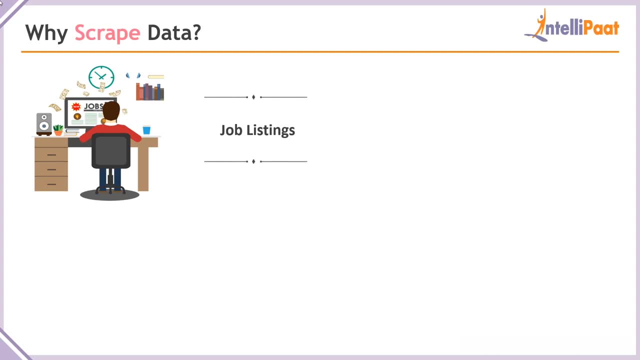 Right. So if all of these job listings were probably put in a very structured Excel sheet, or if these were, you know, put in a very nice place all in one. So if all of these were put in a very nice single place where you can look at, analyze, assess and basically apply, that would be really nice as well. 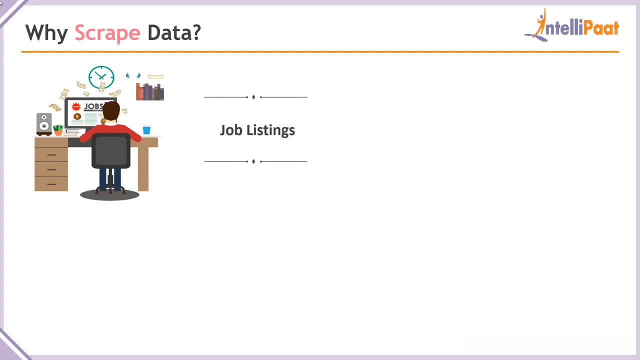 Right. So basically, to perform this, you will require data scraping And you know this is- this is actually a very good example of projects in case you guys want to consider. you know, doing your own projects with respect to jobs, Right. 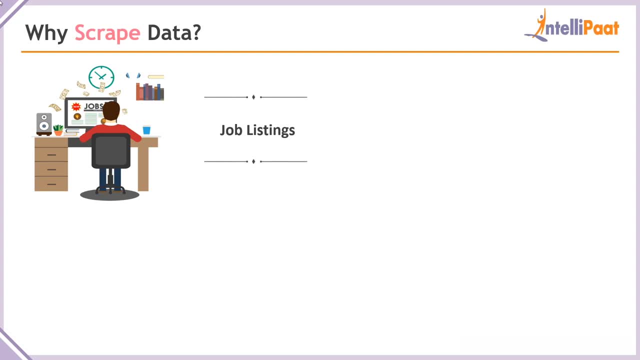 You can do your own projects with respect to job listings as well: Find a keyword, find a career and basically scrape data off various websites where you can create your own list of these jobs available as well. Anyway, coming to the second reason of why one must scrape data, 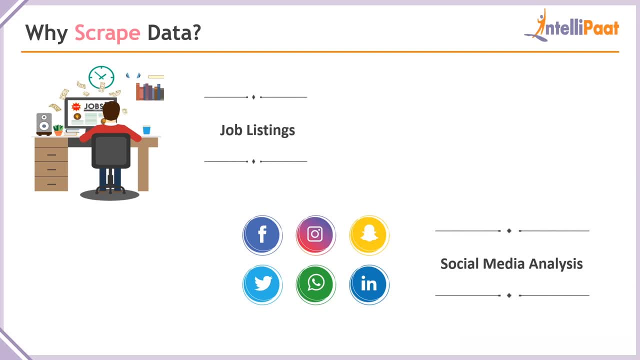 Think about social media analysis. See, all of us pretty much use a minimum of- well, let's say, four out of six social media that you see on your screen Right- Everything from Facebook, Instagram, Snapchat, Twitter, WhatsApp, LinkedIn and more. 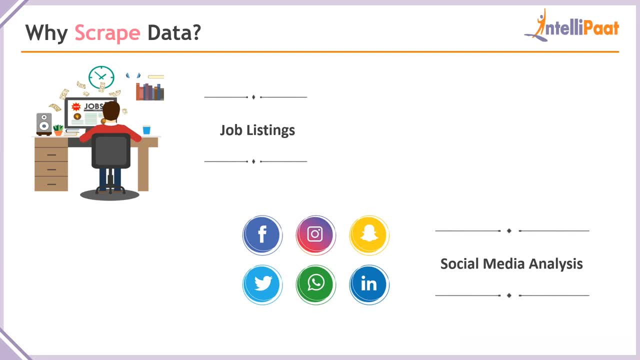 If you are a business person or if you are a marketing enthusiast, come programmer or whatever it is. if you're looking to scale your brand, if you're looking to you know, sell your products more and ensure how your outreach is. as we discussed previously, you will need social media. 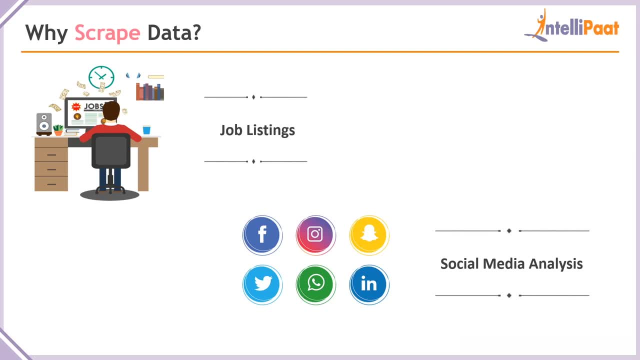 At the end of the day, social media is something you know. we all go back to on our couch at the end of the day to scroll through to see what's happening in our friends life. Well, let me tell you, it is way more than that, because, with the help of social media, brands are being established. 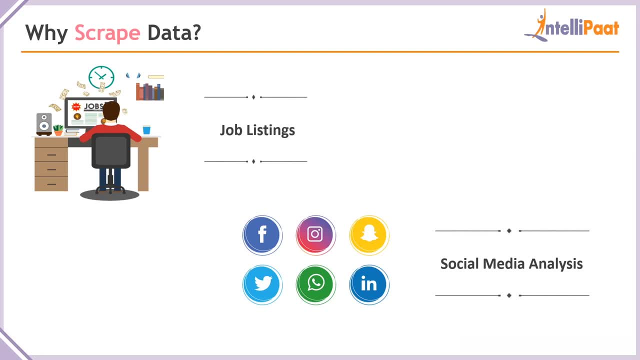 You know they are taking over, They are taking off. So in this competitive world, it is enough that you know people have to start using these tools to help market their brand, to make sure that you know more customers are coming in and whatnot. 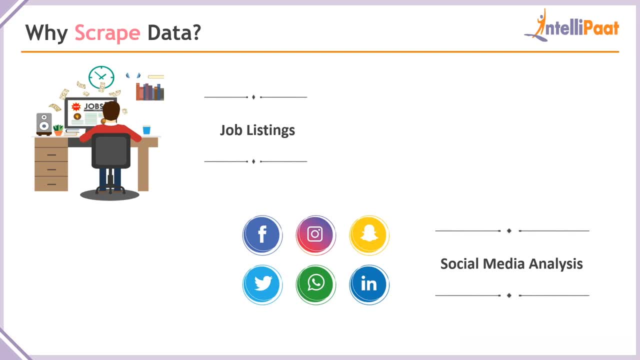 This is one aspect of it. The second aspect of it is that you know you need to understand what your customers feel about your product. You need to understand what your customers, you know, have the opinion about your product, because you know what? three people might be really happy about your product, while 10 people might be showing a disinterest or saying that your product is bad. 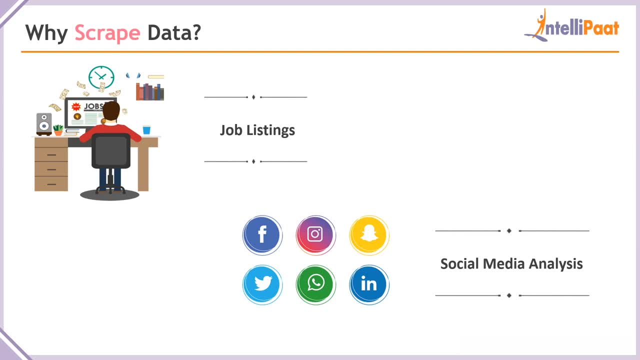 Knowing this can help you with your brand and much more right. So scraping data with respect to social media is very important, not only in terms of businesses, but in general as well. Now, coming to the third reason of why one must perform data scraping is understanding market value comparison. 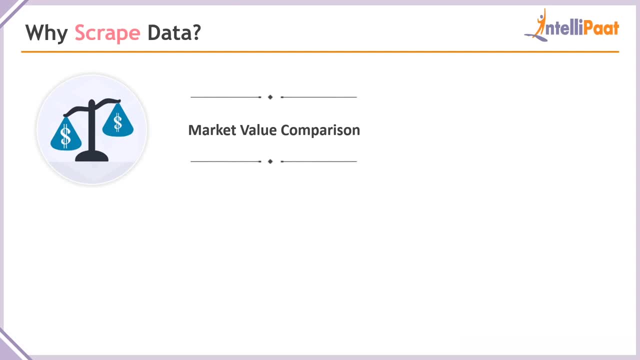 So this is exactly what I was talking about when I gave you the Amazon Flipkart example. So you can. it's not just e-commerce websites, It can be the comparison between any two products. If you're looking for a product you know, you can do that. 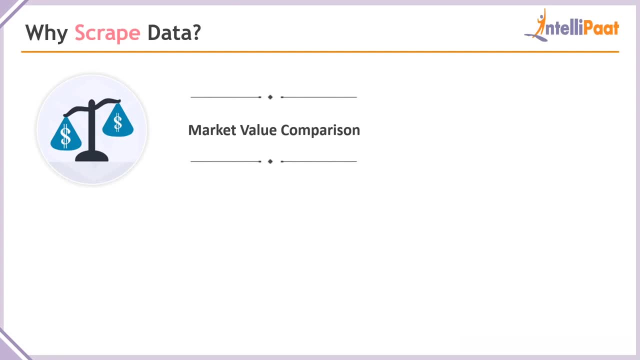 You know- you can bet on it- that there are multiple vendors for the same product. So you know it is very, very rare cases. You know it is 0.001% of cases- where there is only one vendor for your product across the entire world. 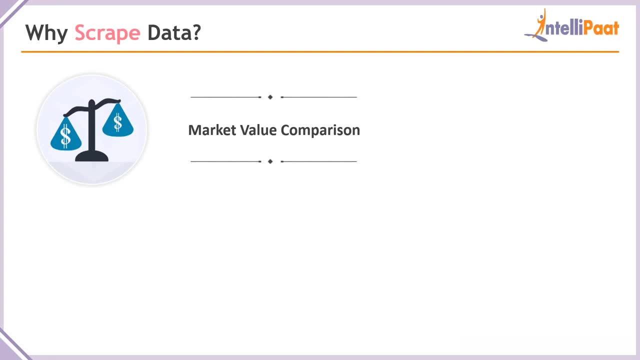 Well, let's talk about the other 99.99 cases, right? So there you know, you have more than one provider who's giving you the product that you're looking for. So in that case, you need to understand, you need to perform analysis to see who's giving it for a lower price. 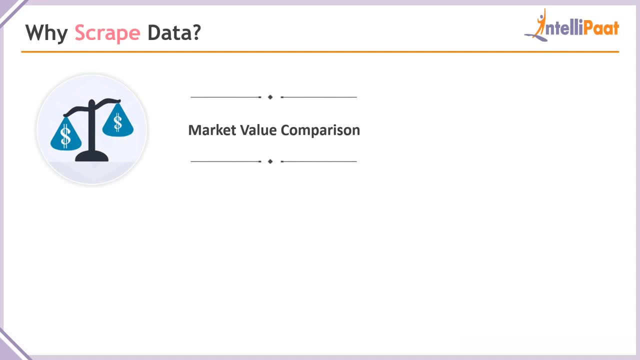 Because if it works out for you at a lower price, you're at an advantage, right? So probably this wouldn't matter if you have a low investment of, say, $1,, $10 or maybe $100, depending on how much you can digest. 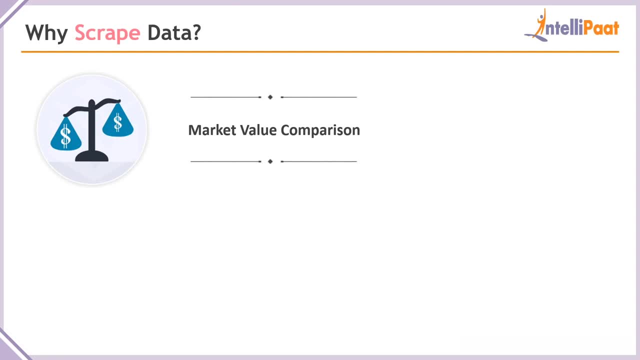 But then if you're looking to purchase something in the thousands of dollars range, probably in the millions of dollars range, then of course this is going to add a lot of value because, again, your savings are in the thousands as well. right, 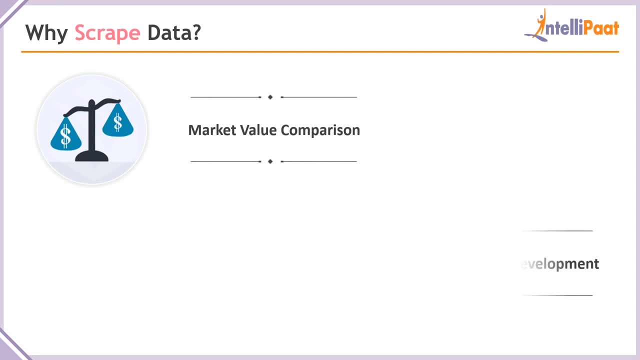 So scraping data for market value comparison is very important And, of course, research and development. When you're understanding that you know, let's say you can provide. you know provide scientists or you know physiologists and everyone in the field of science more data where you know. 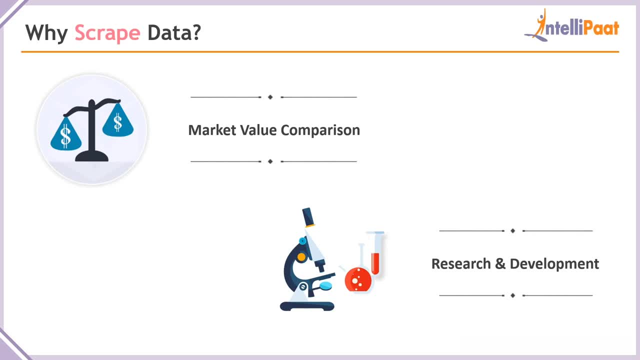 that can be helped, for them to perform analysis and give them, give them a look at the data that pretty much that they've never taken a look at from the angle that you can provide with the use of web scraping is something which is very vital as well. 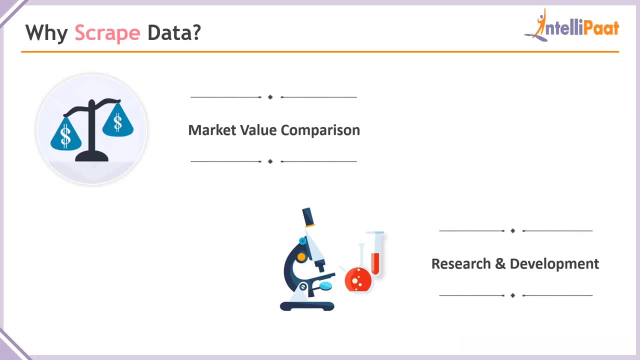 Because you know they can be working with a lot of data. But then once you, once you step in with web scraping, once you give them data, it might provide them the angle, It might provide them some clarity, It might provide them basically what I'm trying. 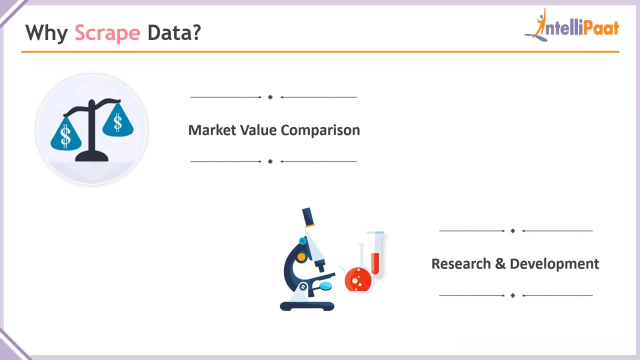 So, basically, what I'm trying to tell you is that you know it will provide them with a view that they have not thought of looking at as well, And, of course, all of these data can be further put into use by making use of artificial intelligence. 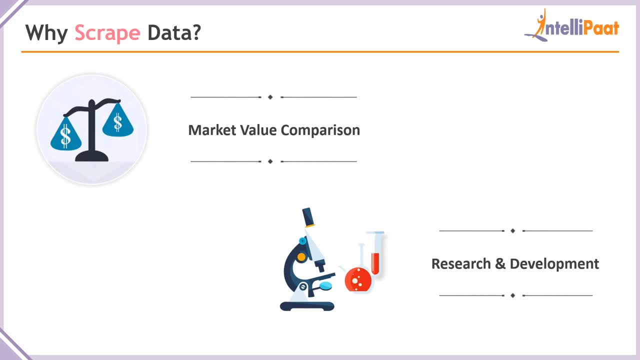 machine learning or whatever it is, But then to get to that, you need to give them the data right, And this is exactly what and why it's important to scrape data for the world of research and development as well. So, on that note, you might have a question asking saying: 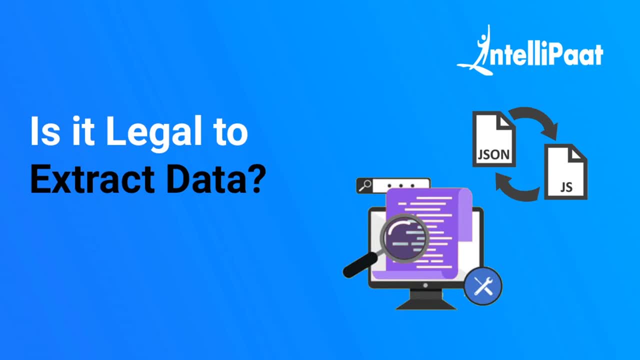 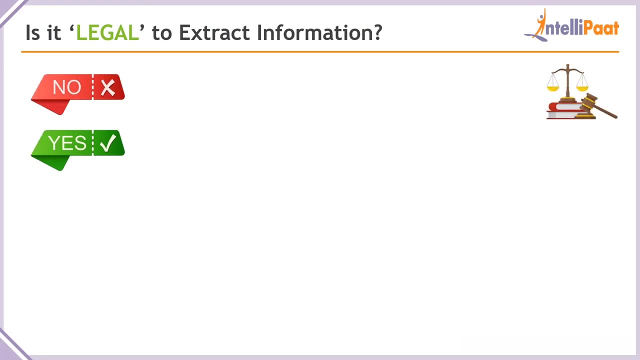 is it legal to scrape data? Is it legal to start pulling data from everywhere around the world? Well, to answer this is a bit tricky. I'll tell you why. The answer is yes and no, So you can legally extract some information from websites. 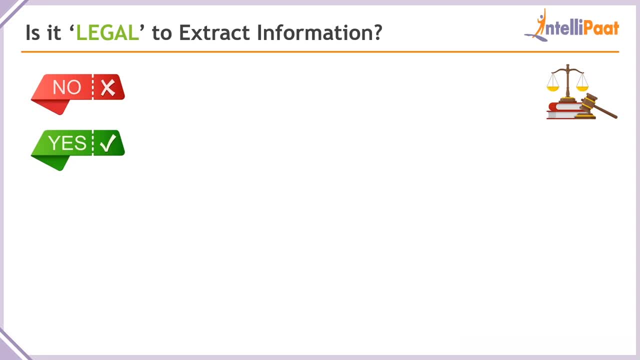 And you can, of course, you know, illegally- do it as well. So to understand how you can, you know, abide by the laws to make sure what's legal to be pulled, what's not legal to be used. the websites will actually tell the users about it. 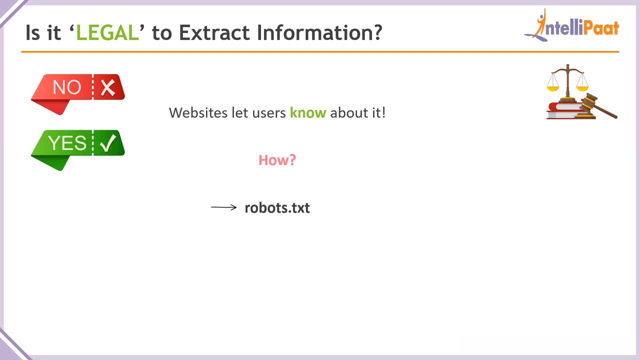 So you know the websites will tell the users saying, hey, this is legal to do, This is not legal to do. So how, You might be asking. you know how are the websites telling the users, Because you don't see it anywhere on the websites, right? 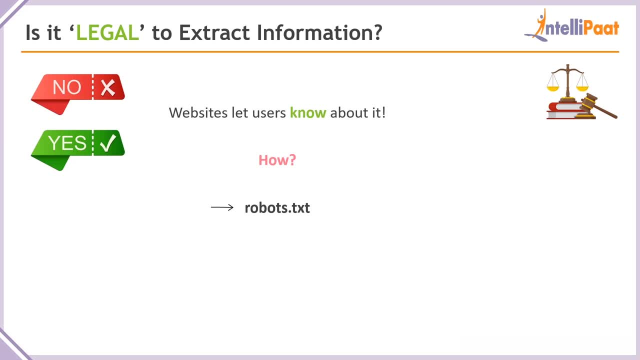 So every website has a file called as robotstxt, And this robotstxt will basically tell all these crawler robots, all these spider robots which basically go on to you know, pick the actual data from the websites, saying hey, you're allowed to do this. 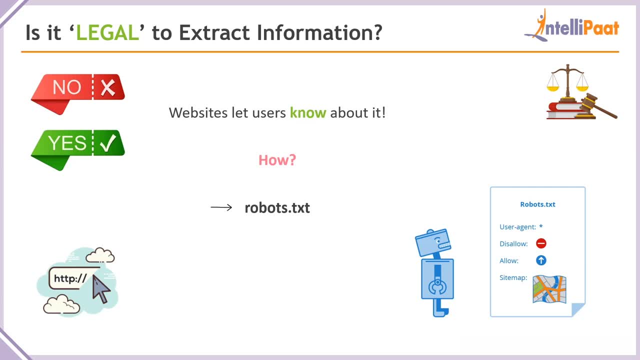 You're not allowed for this particular information. So when these websites say, and these robots, basically, when they you know, they can have all the access they want to everything that they're allowed to And once if someone with a very bad intent tries to, you know, pick up something. 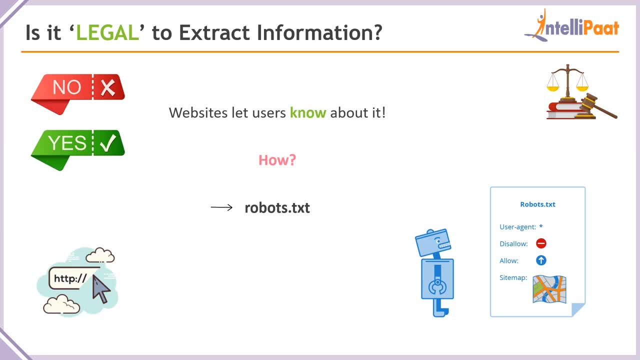 pick up information from a website which is not allowed to access, then you know their intentions are not good And you know they might be doing something with your data which they're not supposed to. So you know, let your access is basically amazoncom slash robotstxt. 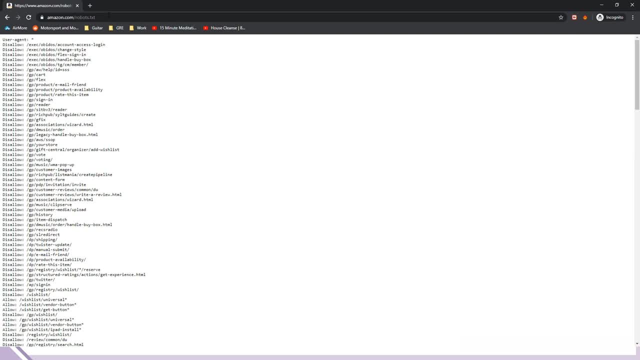 And as soon as you hit enter it will take you to their file. you know where. they will tell you what you can allow and what you cannot allow. So you can see disallow, slash wishlist. So all of these pages which start with disallow means that you cannot legally access all of these as well. 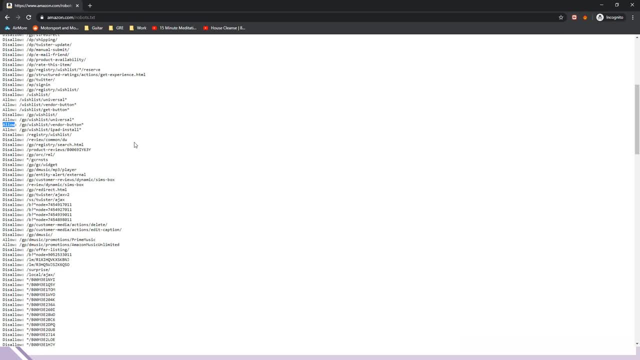 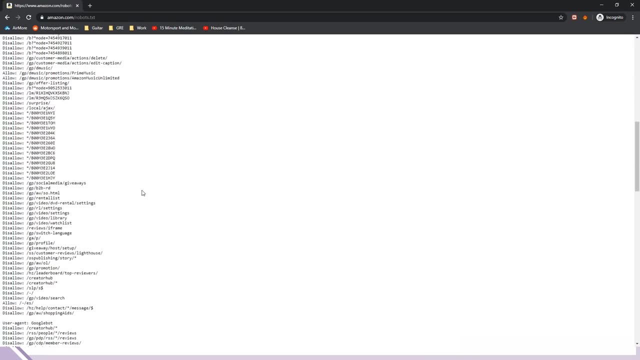 You can see allow as well. So, basically, allow will tell you. hey, you know what? You can have legal access to all of these as well. So this is exactly what I was talking about, But then, to give you more clarity on what this means, it's not just Amazon. 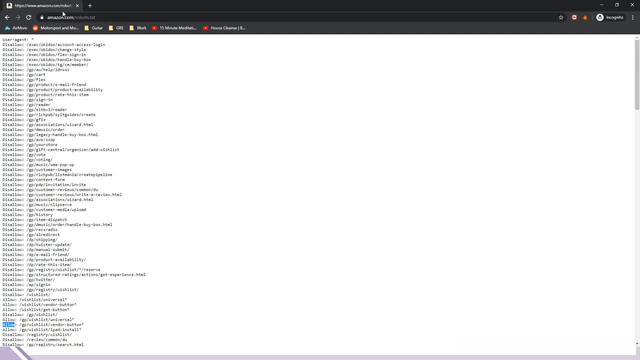 You can visit any of the websites and just type in slash, robotstxt, And this will give you an understanding to see if you can actually- you know- scrape their data or not legally. So, in fact, to add value to my point, here is what it would look like. 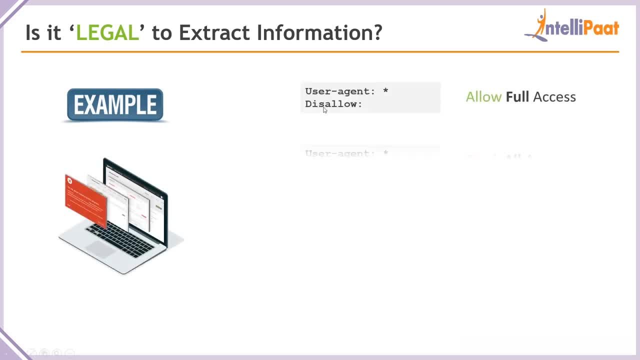 So, basically, you know, as I mentioned, any website will have this file And this is what it basically means. as soon as we saw User agent start disallow- If disallow is not followed by anything, it basically means that you know the user, or the crawler robot or the spider robot. 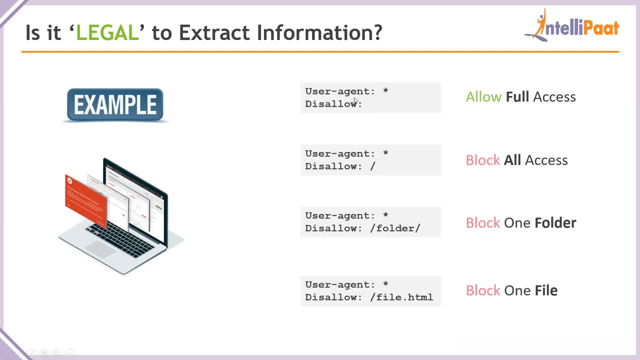 basically, which is going to pick the information for us? it has full access to their website And if we have a disallow and if you put in a slash there, it means that it will block all access And you know, no data can be scraped from that. 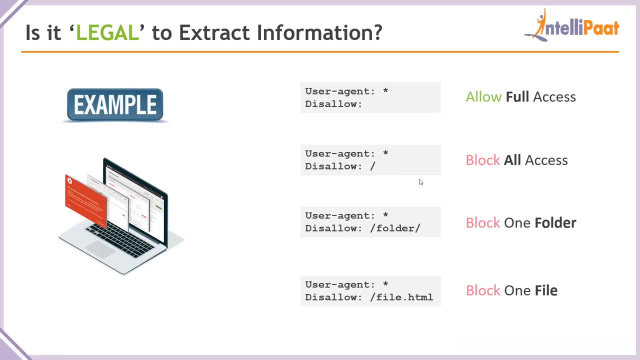 But then you can actually prevent access to particular folders. You can prevent access to particular files and much more. So you can see disallow slash folder slash. This means that this one particular folder has blocked access And you know you cannot access this when you're pretty much trying to scrape the data. 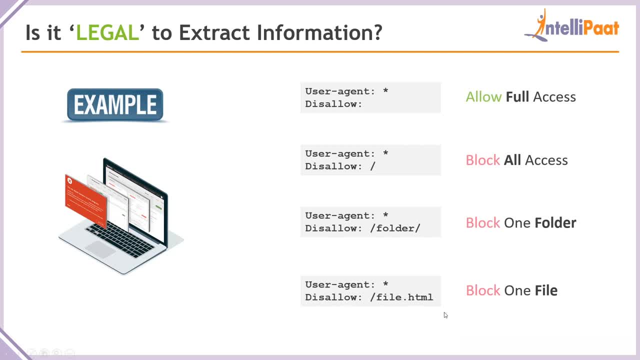 And then there is a disallow slash file dot HTML, And this ensures that you know there's no data. There's one particular file which is basically blocked for access by all of these crawler robots as well. So this is very important for you to understand, even before you begin scraping data off the Internet. 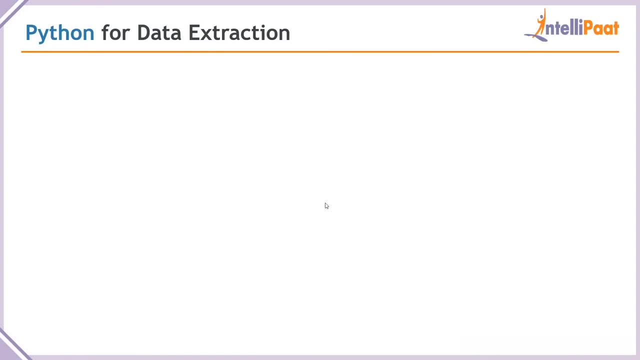 And now the question comes: Python for data extraction. what makes Python the tool that one must go on to use? The first thing when we talk about Python is ease of use. So Python has been this amazing language and personally, you know, been a fan of it, been using it for multiple years now. 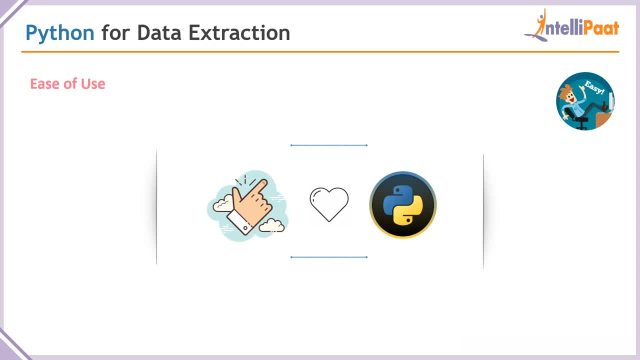 Seeing it take over the top position when you're comparing it with Java or whatever it is. Python is amazingly easy to work with. There are multiple reasons. One, it's very readable for people who have never used Python before. Two, the syntax is again very easily understandable. 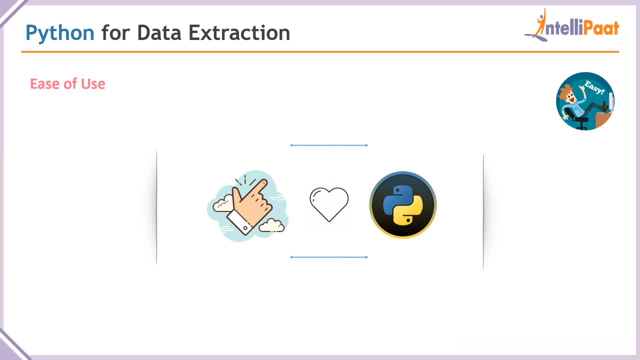 And you do not need you know a lot of training when you're working with Python. Of course, structured training is very important to understand the core values of Python and how you can go to use it effectively as well, But the point here is that you know there is no semicolons. 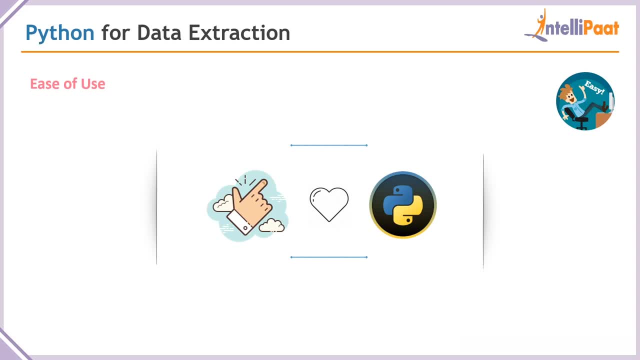 There is no complex syntax And everything at the end of the day is a breeze when you're working with Python. So of course, I think many people in the comment section can agree to this point on how easy Python is to use when you compare it with all the other programming languages out there. 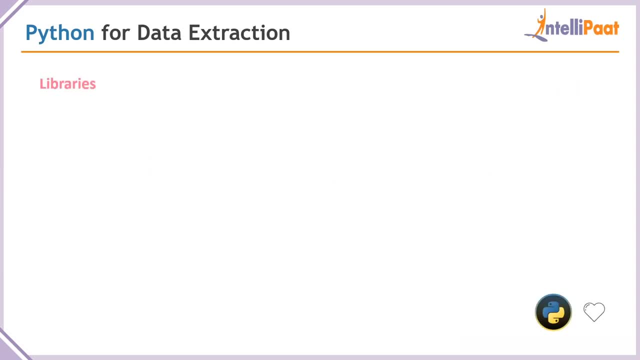 So point number two is something very important. Point number two is what makes Python what it is. It is the number of libraries that you know Python supports. See, for example, in the world of data extraction: we will perform computations, we will perform, you know, data storage methodologies. 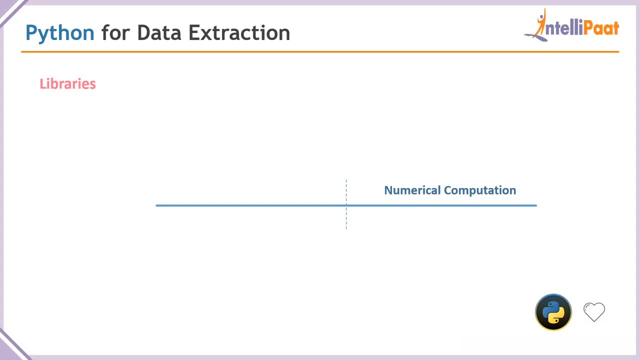 and we will go on to visualize this data at the end as well. So, for numerical computations, you have libraries such as Panda and NumPy, which will perform any computation on the data that you have extracted, And for data visualization we have tools such as Seaborn, Matplotlib and much more. 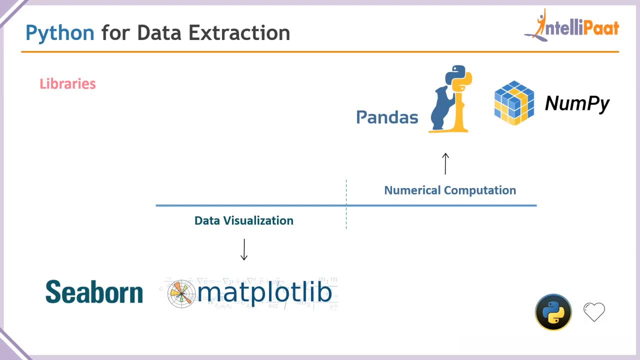 which will basically help you even after you have achieved the results of data extraction as well. And these are just four libraries among hundreds of libraries. There are hundreds and hundreds of libraries that are present, which are being used around the world as we speak. 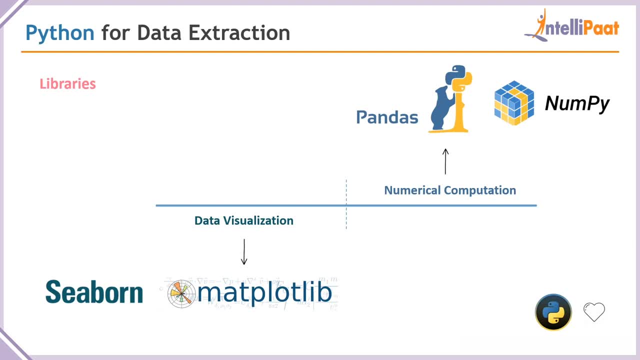 basically, which makes what Python what it is, Because, at the end of the day, with getting access to so many open source libraries, you know you're part of a huge community and you're using tools which will make your job a lot easier. 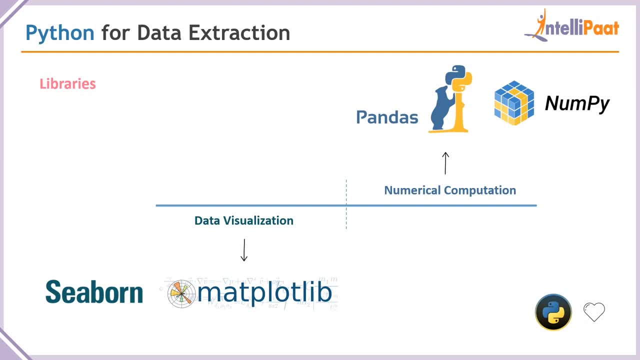 Be it data extraction, be it machine learning, be it neural networks, whatever it is, with respect to Python, it just makes it easier, And this adds value to my last point as well. So, coming to the next point, it's small code. 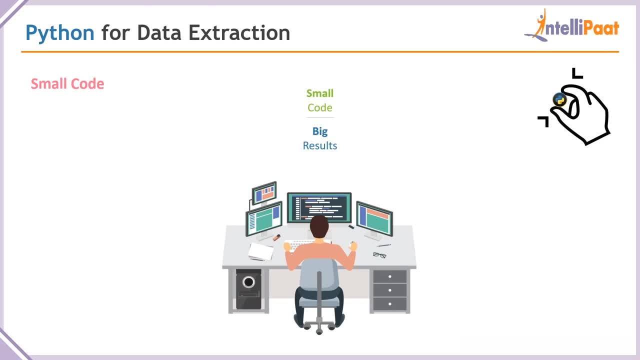 You might be wondering what I say by small code With respect to Python. you know, as I mentioned, the syntax is not complex. One more thing is that the syntax is not long. For small amounts of code, you can basically get big results. 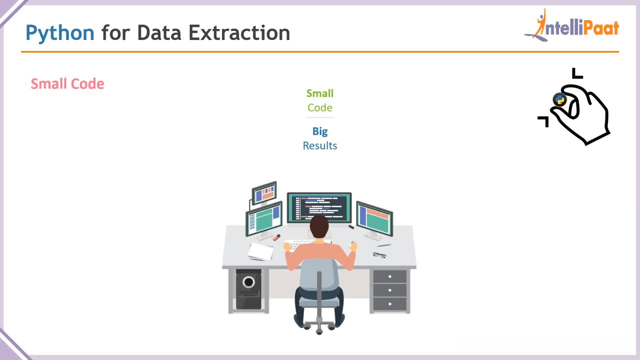 In Java, if you have to compare to, you know pretty much: go on to print a hello world. you have to write four or five lines of code. Those are complex syntaxes as well. So for a beginner who has never seen programming before, that will be overwhelming. 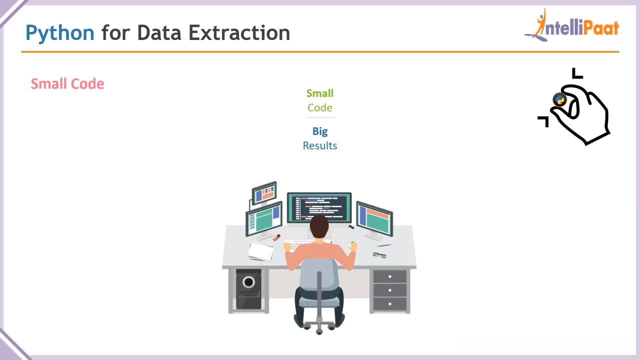 With Python. it is pretty simple. It says: print, open your braces, put your message inside and hit enter, and your results are printed. So I just gave you a simple example. Again, even with respect to data extraction, you need to understand that. you know there is a small amount of code. 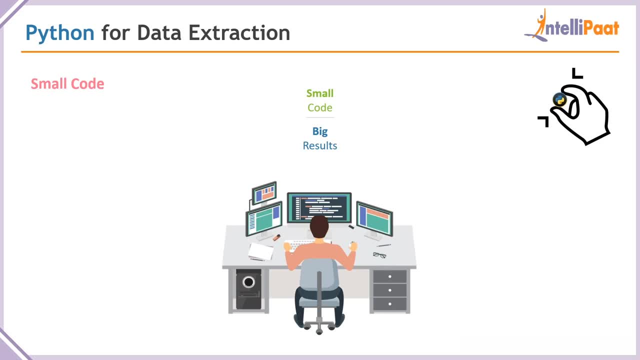 But, at the end of the day, the results that you get for typing the small amount of code is huge, And this, in my opinion, is one of the most important aspect of using Python for data extraction as well. So, coming to the next point, it's again a very nice point. 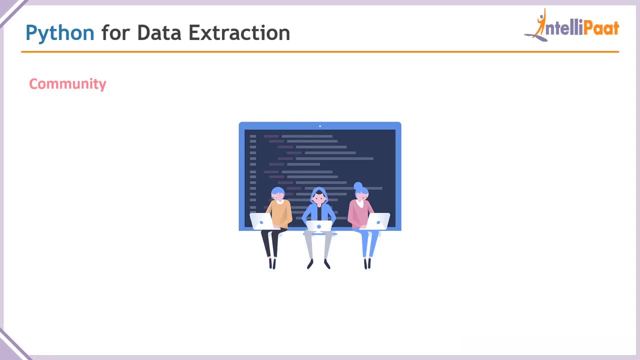 Here is that it's the community When you're working with data extraction or any other concepts with respect to Python. we have an amazing open source community where you know everyone is friendly, Everyone wants to help each other out and pretty much you know develop products, establish brands, whatever it is. 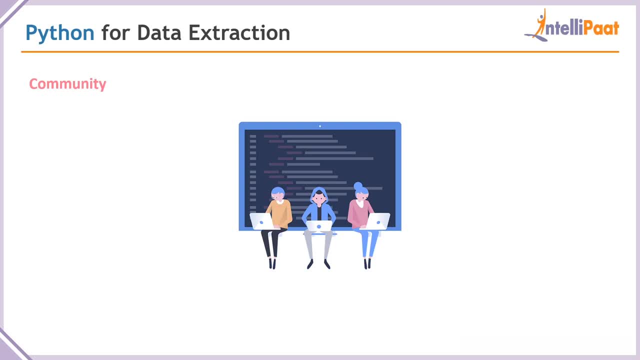 Everyone is very friendly And this entire community is filled with people who are enthusiasts, who are willing to help each other out and who are basically willing to see that you know. all of them grow together In the world of programming as well. 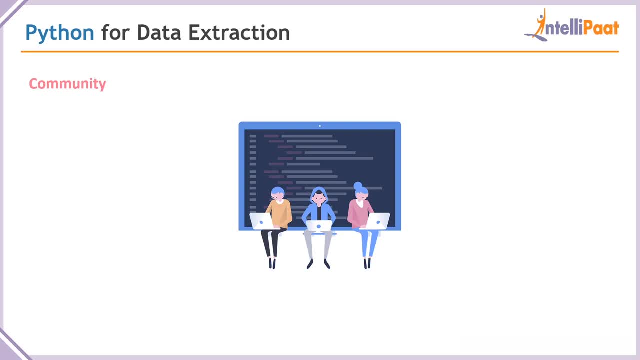 So this is why, personally, I love Python too And, again, I am sure you know our viewers can agree to this point as well. So you might be wondering: what are the Python libraries available for data extraction? Well, there are many, many libraries, but then here are the top three most used libraries: 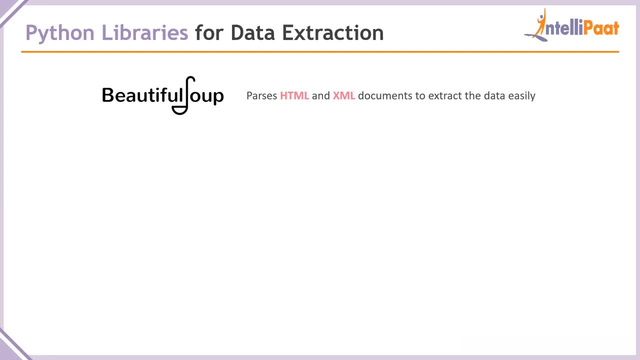 The first thing is Beautiful Soup. So Beautiful Soup is again another open source library which basically parses your HTML and XML, you know documents- and makes sure that you know you can extract all of this information Very, very easily. 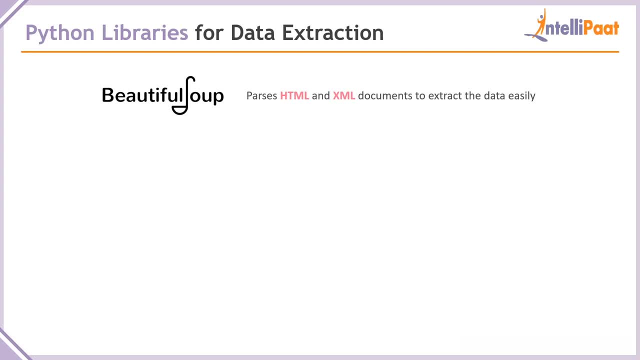 So you might be wondering what parse basically means. So parsing is an operation of performing syntactical analysis, where you're trying to make sense of symbols, where you're trying to make sense of the text which is given, the strings or whatever it is. 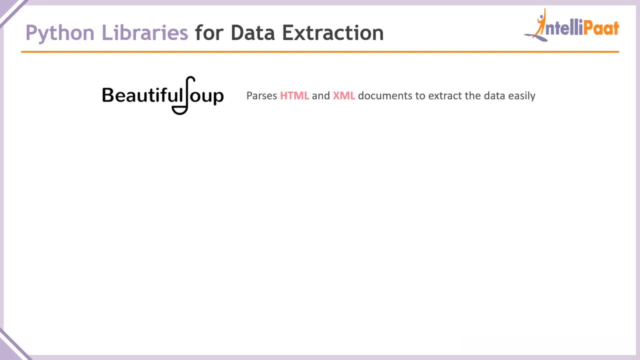 And then you know bringing you that information So Beautiful. Soup again is a very widely used Python library for data extraction alongside Selenium, So Selenium is basically used for automating your browser activities as well, So when you perform web applications. 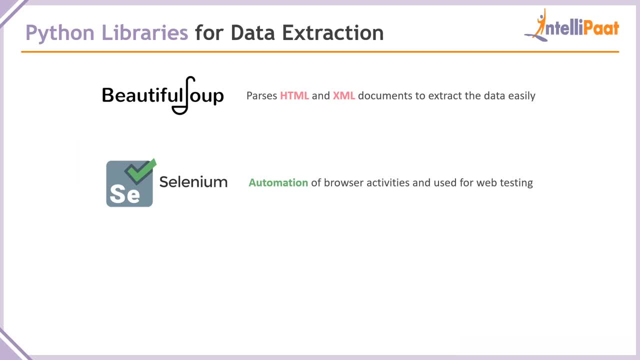 web testing. when you perform activities where you're, you know, pulling the data continuously, you have to go on to test to see if your data is being pulled right, to analyze your data to you know. automate this process of verification and validation. 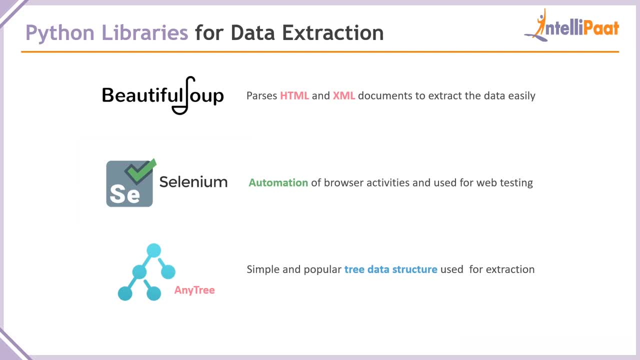 So Selenium is used right after Beautiful Soup for that. And then there's AnyTree. AnyTree is basically, you know, helping you create a tree data structure which is used for data extraction. So a tree data structure, at the end of the day, will basically make sure that you know your data is organized. 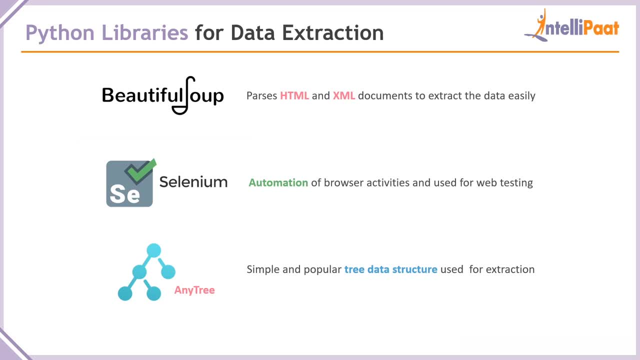 and it can be pulled in a structure. It can be pulled in a structured way And this will help in further analysis, in further storage and much more See, there are many other tools you can use as well. There is a request which you can use. 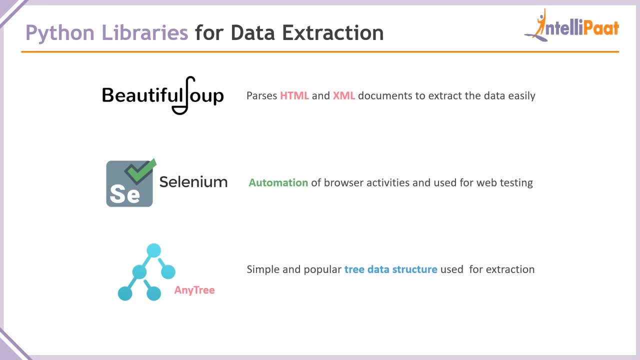 There is LXML and there is many other tools as well, But these three are mostly the top used tree because one: we are talking about converting your data into something useful. The second one: we are basically pulling the data for AnyTree to use. 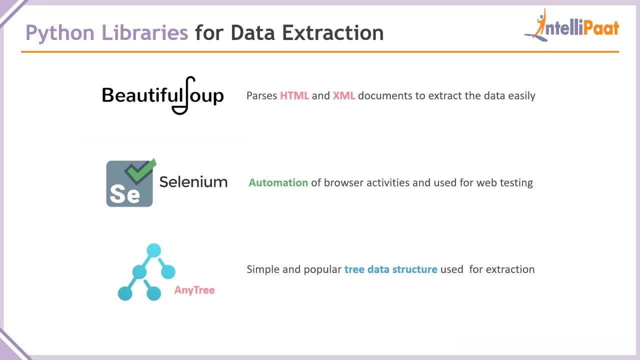 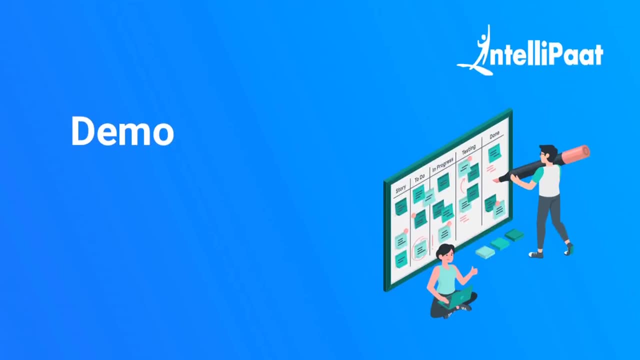 And after that, you know, we'll be using Selenium to basically test and automate the process as well. So, as I just mentioned, you know there are multiple libraries which one can go on to use for data extraction, And this quickly brings us to the demo, where we'll actually get to see this hands-on. 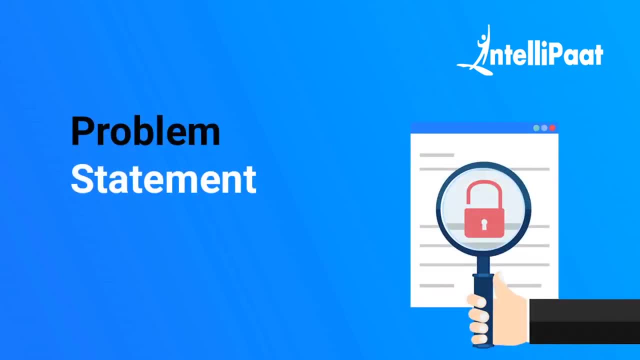 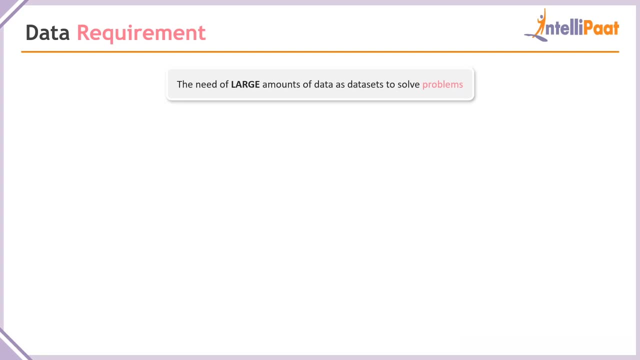 And just before we, you know- jump to the demo, we need to understand the problem statement at hand. So what is the problem that we are facing in today's world with respect to data? In my opinion, it is data requirement, Because, see, when you're basically trying to solve a problem which needs a lot of data, 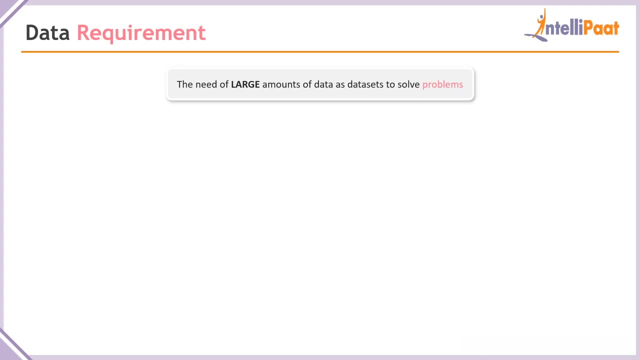 first thing, you need all these data to work with right. So here is where data extraction is a king. When you're working with data extraction, you can have the ability to basically provide all the data that's required, For example, for the creation of data sets. 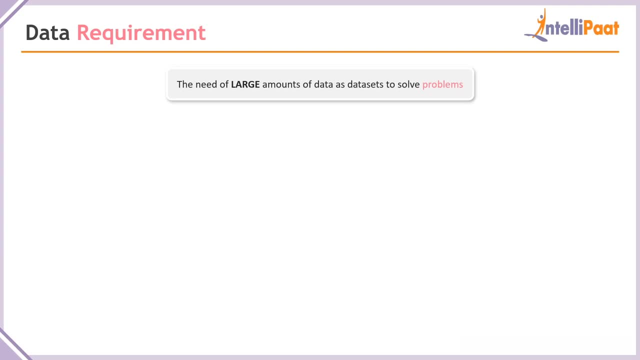 And these created data sets will help solve the world's problems, right? So let me give you an example. When you're working with artificial intelligence, machine learning, neural networks or whatever it is, more the data you provide, there's a good chance that your machines and your neural nets, or whatever it is- 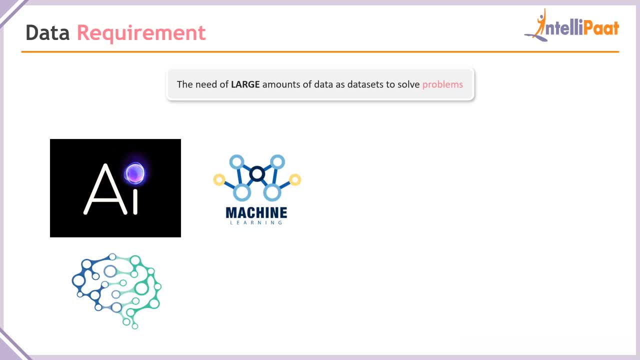 it will learn better and understand better, Understand quicker. So it's not only about artificial intelligence that you know. more the data, better the learning, But when you talk about any other situation as well, you know, if you were given price comparison of products from just two places, would it make more sense? 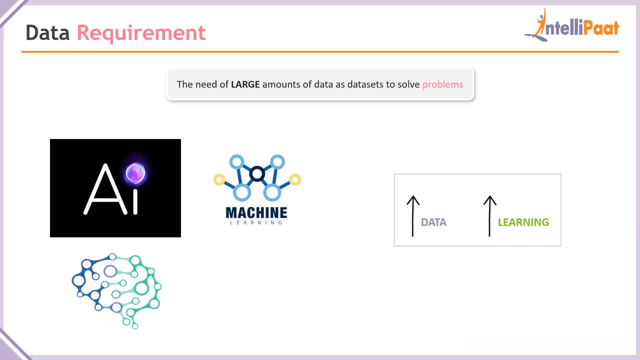 Or if I could give you a price comparison of 10 places. the 10 places would basically be a better, you know- point of reference for a business decision. right, Exactly my point here. So more the data, better the learning, better business decisions. 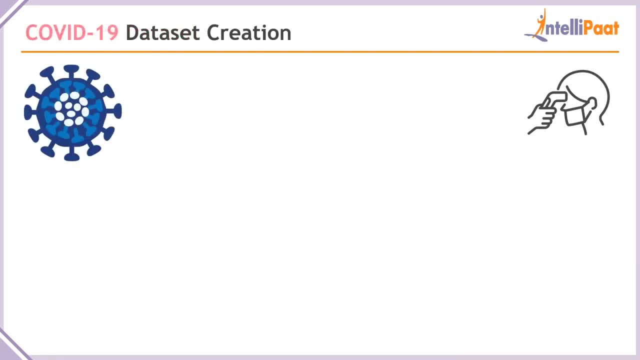 better key performance indications and much more. So let's consider one of the things that's happening right now. So, for example, we have the COVID-19 outbreak across the world right now, And it is something very grievous as well When you look at the numbers on your screen. basically, 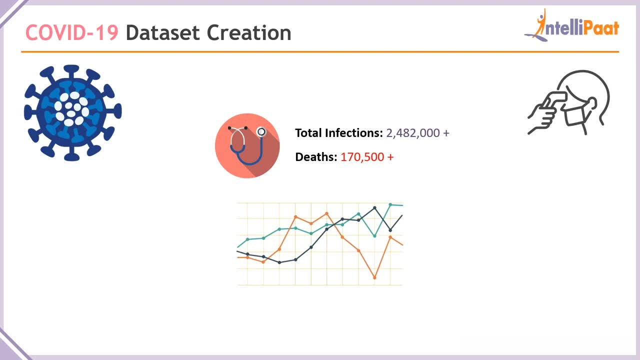 we had total infections of 2.4 million and 170,000 deaths at the time of the creation of this video as well, And pretty much this number is going on and on every single second. It's very scary to see And at this point of time again, I would like to enforce everyone to take all the precautions. 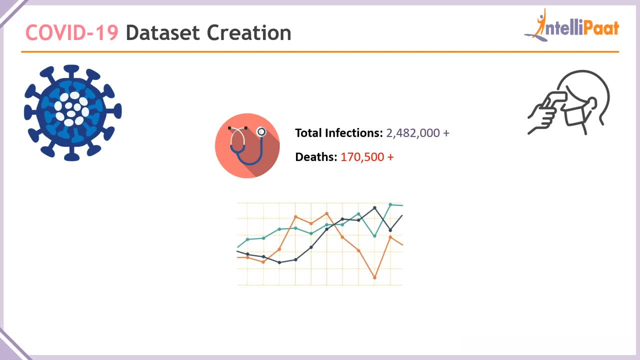 That is, stay safe, stay in quarantine, and you know we can fight COVID-19.. So, basically, humanity has fought multiple viruses across the history of the last hundred years and more. So pretty much you know this is an easy task at hand. 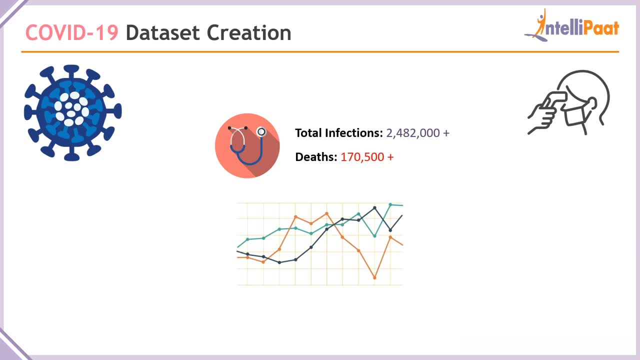 Everyone does their job And you know, let the doctors work their thing. And let's see as IT people, let's see as the people who are computer scientists enthusiasts, IT field enthusiasts, let's see how we can help them out better to achieve this right. 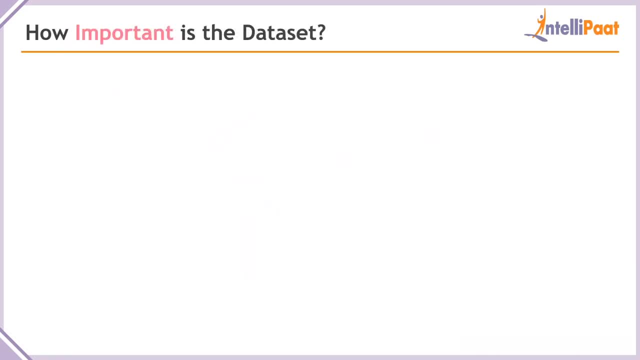 And that's exactly my point here as well. So again, when we're talking about how important is a data set to solve a problem, let's see if we can, you know, bring machine learning together and medicine together. So we have a comprehensive video on the channel. 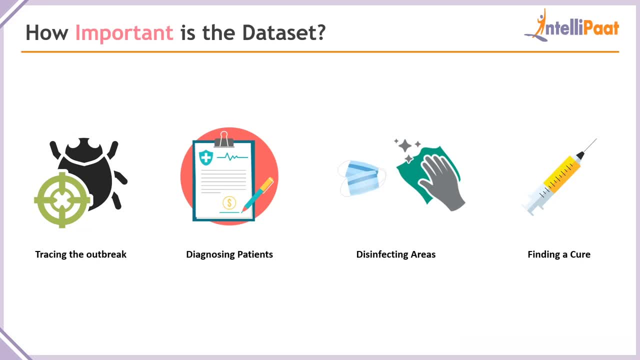 which will guide you on how machine learning is basically used to fight against COVID-19 as well. So make sure you check that out after this video. So, coming back to how important the data sets are, the first thing your data set can help in this particular case. 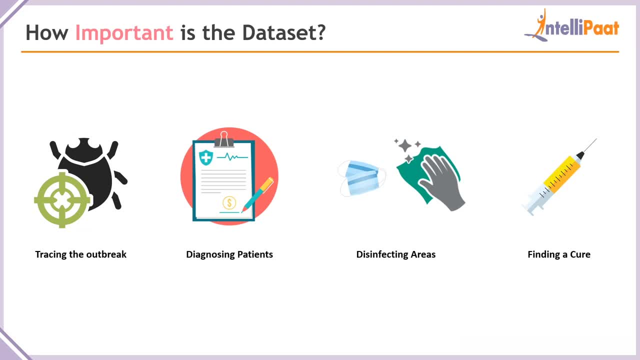 it'll tell you where you can trace the outbreak, from where it originated, how it started out, where is it spreading, how quick it's spreading and much more. Diagnosing patients is something very important Again. it'll help you tell you know what patients have been diagnosed at what time. 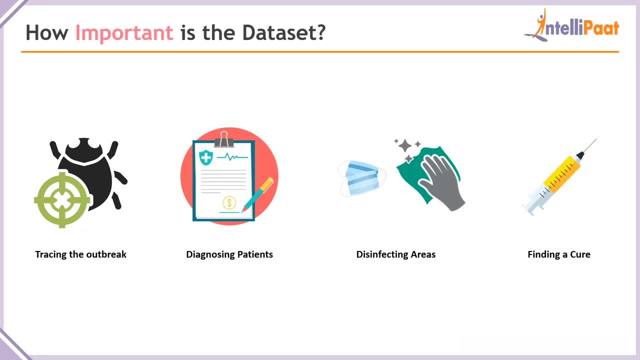 for what particular disease or whatever conditions. they have as well. Disinfecting areas: you can find out by making use of machine learning models saying where the contamination is highest and help disinfect those areas as well, And then when you're looking at finding a cure. 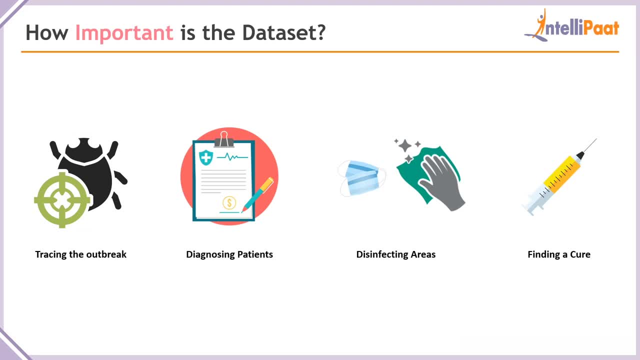 probably this is the most important thing. This is the most you know widely asked thing right now: to see if computers can help fight against the virus. And of course, computers are doing everything they can. There are experts out there who are bringing together the world of IT and medicine just for this cause. 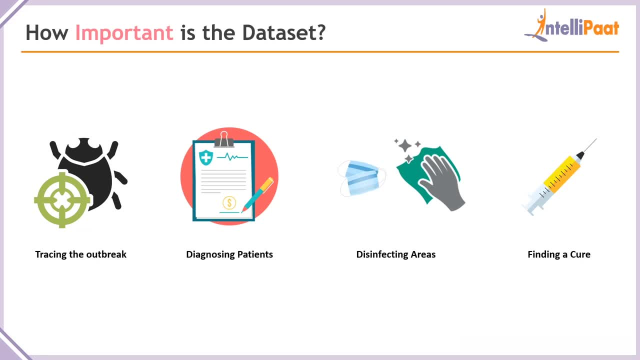 So if computers can help- you know scientists- find a cure for this particular disease, it would help. And again, if we take a quick backtrack, of course medicine in all of its glory could be the one finding the cure, But then the field of computer science? 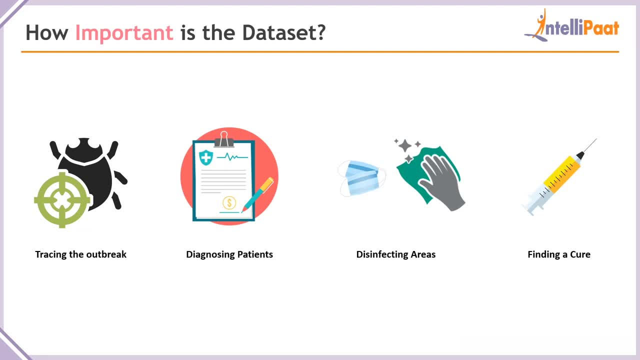 if it can speed up something in the field of medicine. that is what we're basically achieving. To speed up something, we need more data again, and more data is obtained by making use of data extraction. right, So you see where we're going here. 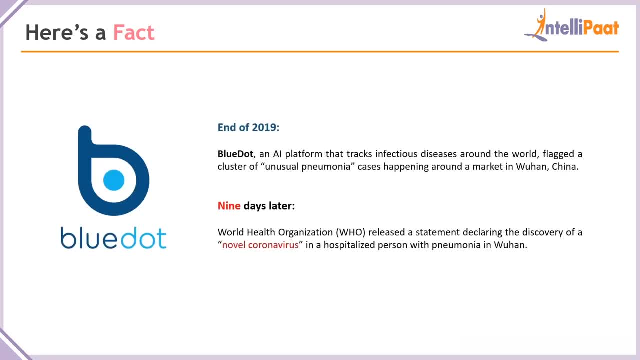 So, just before we dive into the world of showing you how data extraction works with respect to the demo, here is a sample fact about how machine learning came into picture. So, basically, Blue Dot is an artificial intelligence platform which basically tracks all the infectious diseases that happen, right? 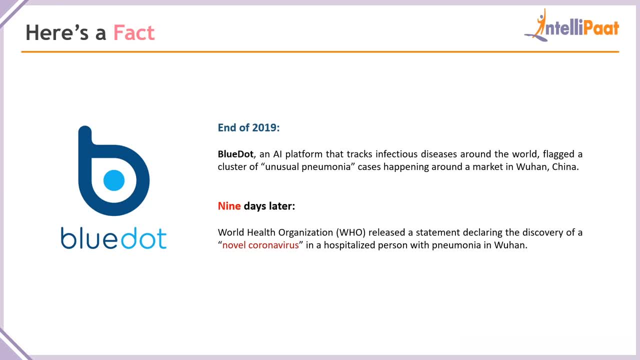 So this actually found out that there was a lot of pneumonia cases happening around one particular market in Wuhan, China, And just nine days later, after the Blue Dot platform found out this unusual rise in cases, World Health Organization stated that they have found a new virus out there. 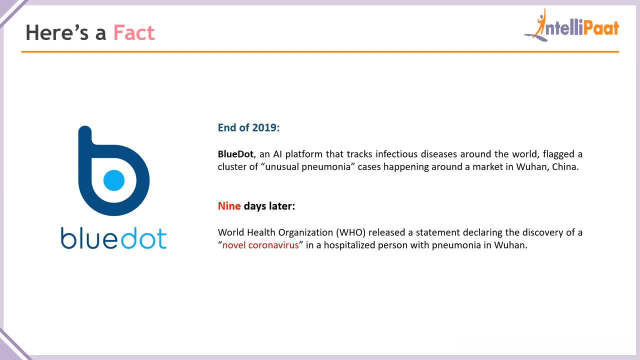 And you know, there are a lot of people hospitalized with respect to pneumonia as well, And this was at the end of 2019.. And now we know that in the April of 2020, we know where we are. we know the 100,000 deaths which has happened. 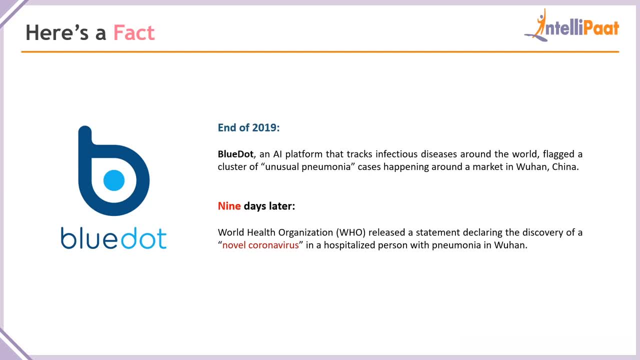 2.4 million cases and whatnot right. So this again was one of the places where IT helped And it could only do this where if it had all the data from around this market, in Wuhan or whatever, it is right. 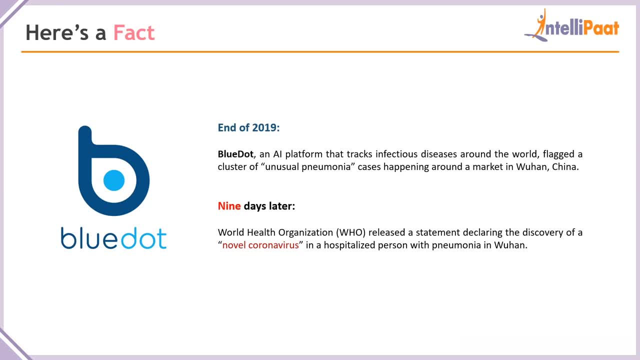 So again, they and the people at Blue Dot basically again made use of data extraction to get all of these data and create artificial intelligence models around it And then, you know, put out a conclusion saying there are a lot of pneumonia cases here as well. 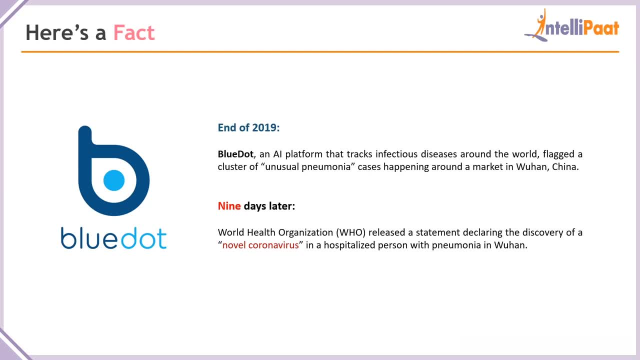 So this is exactly one case I mean. so I picked up a medical case study to show you guys because, again, I believe that artificial intelligence, I believe that you can make use of machines with medicine together to help speed up today's world of medical research and whatever it is in general. 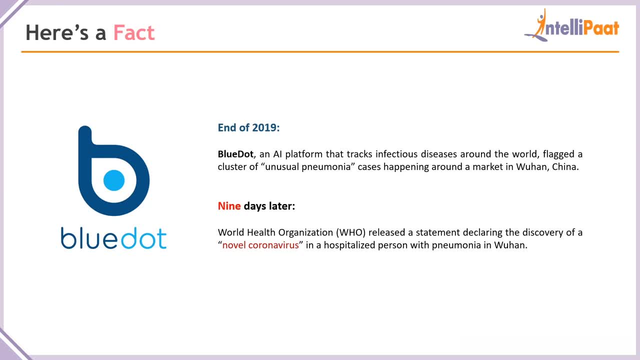 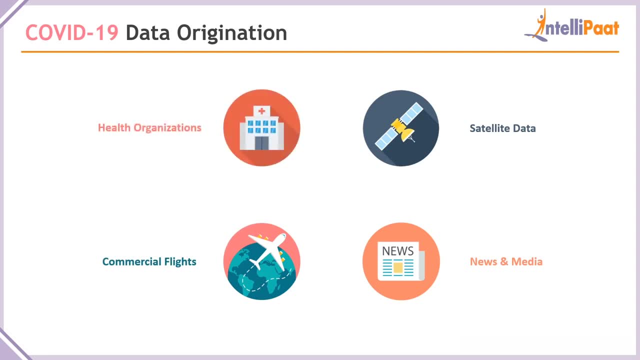 So I'm a huge fan of that And I hope you know you guys could see the connection as well. So, coming to where you can pick up the data, in our case, let's say, COVID-19, data set creation, you know you can have data picked up from the satellites. 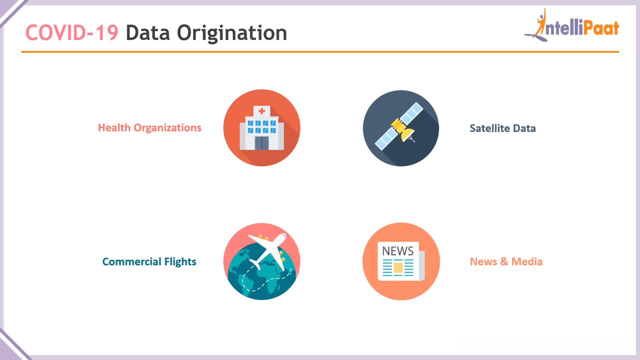 you can have data picked up from the news. You can see who all flew around the world, at what time to trace and understand. you know where there could be an outbreak by taking all the data from the flights across the world And, of course, all the health organizations. 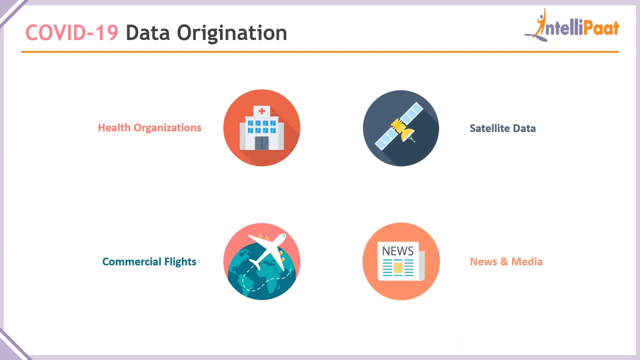 hospitals, your local governing bodies, which is taking care of the local areas as well. So you know there are multiple places where you can find a lot of data. For example, every day you can check out. you know there are news about where hotspots are. 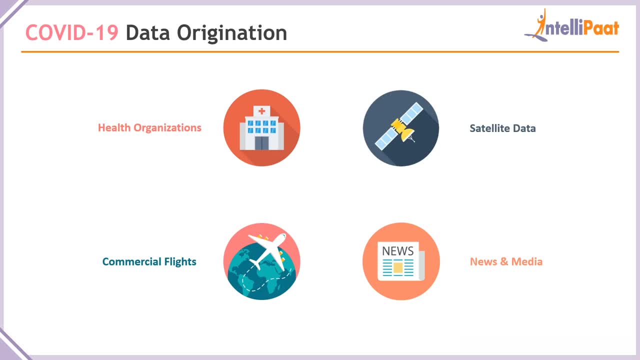 where there is a lockdown, where there is a complete lockdown, Where you know people cannot step out of the houses as well. So when you look at the data, there is a plethora of data. There is a lot of data To go on to use this effectively. 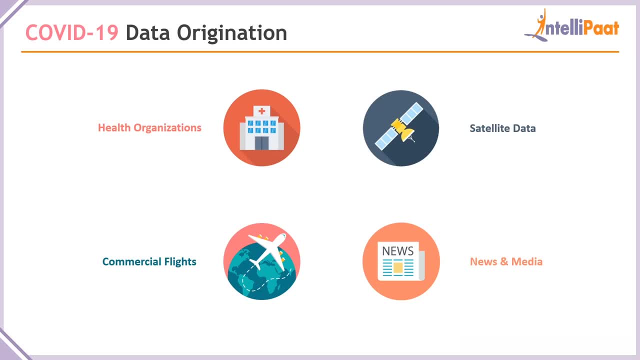 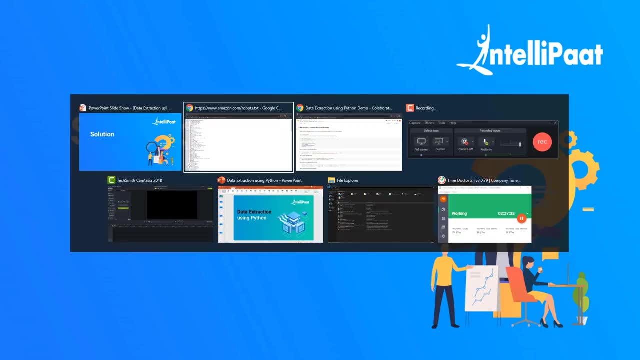 you need to create that structured aspect that I spoke about in the starting of the session, right? So just onto that. here is what the solution would look like: to perform data extraction on a data set such as the COVID-19 data set. 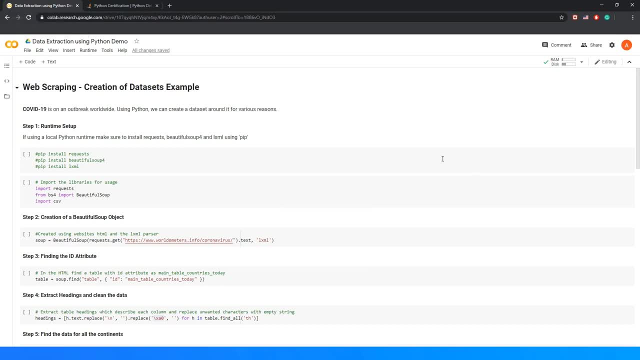 by making use of web scraping, by making use of data extraction. So, as mentioned, we'll be making use of Python in this particular case and we'll create a data set for various reasons And all the various reasons we just discussed in the problem statement, right? 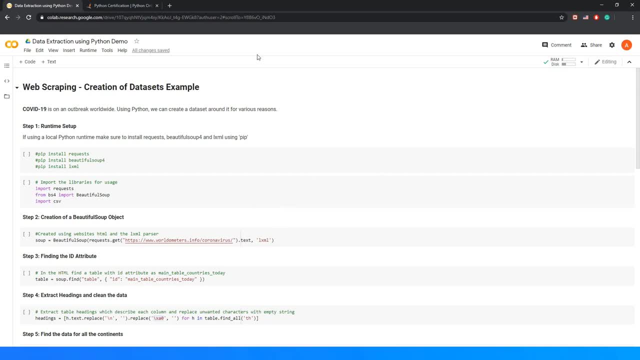 So, quickly coming on to how it works, it is pretty simple. So it's about 10 or 11 steps, and it's really simple to follow as well, So follow along with me. The first step to perform data extraction is to make sure you set up everything you require. 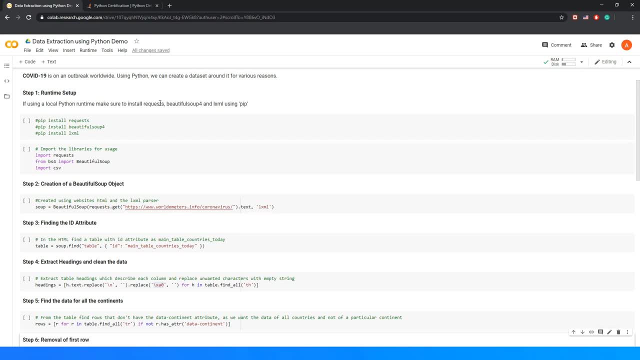 in your Python runtime environment, For example. here we're making use of Google Collab. basically, it's a free Jupyter notebook where you can run Python commands online and everything is, you know, stored on the Google's ecosystem, and they provide you storage and computation power as well. 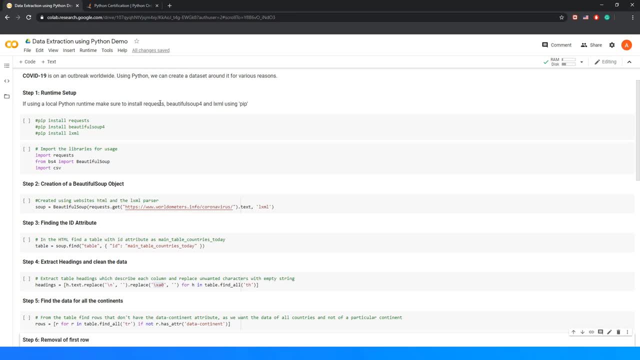 But then you know, I'm aware that most of you might not be using Google Collab. So if you're using your local machine, if you're using any other environment to run your Python code, just make sure you install a couple of libraries. 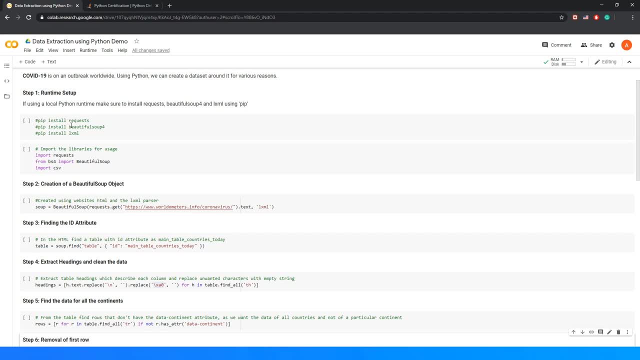 before we begin with, As discussed, you know, beautiful soup4, again is a very important library for web scraping. We have requests as well, So requests will basically help you pull and parse data from the HTML sources we'll be looking at as well. 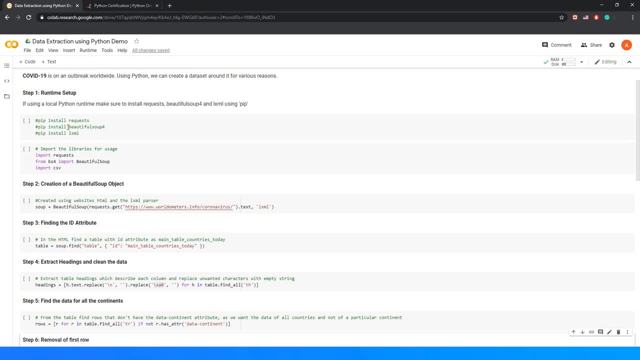 So in this case, we'll be pulling data from a very famous website called as worldometersinfo. So these guys have been putting out very structured information when it comes to how the outbreak is being handled, and all So to do that, to pull the data. 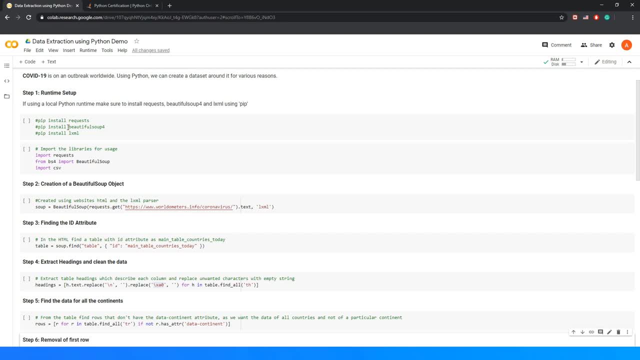 to pull all the HTML data and to analyze and understand it, we require requests And we have a library called as LXML as well. So LXML again will help you parse your XML data and pretty much make it understandable and make it usable for further down the line. 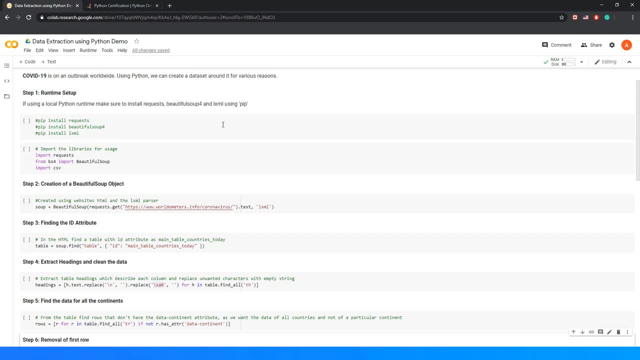 So you can execute these code statements that are in the comments, in case if you're using any other environment as well. So, coming to Google Colab, basically, Google Colab has all of it covered for us, So all I need to do is run it. 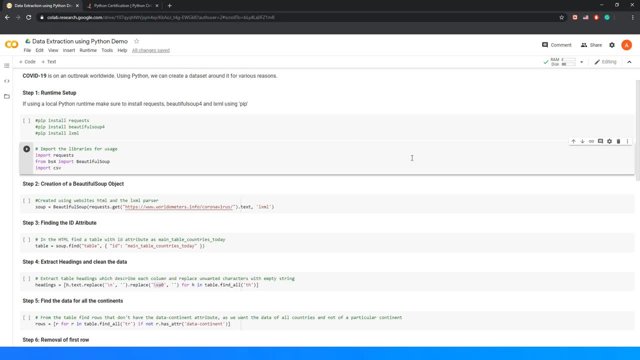 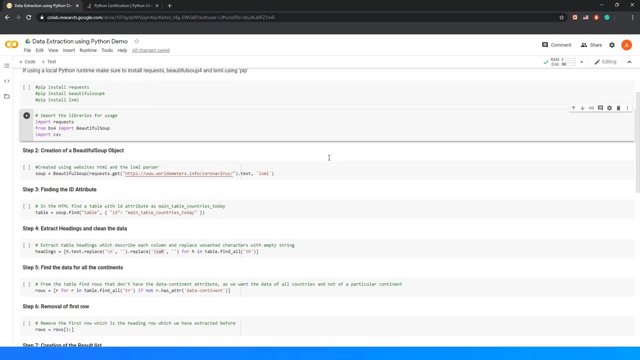 and basically it is imported because it's already installed in the backend. Step one is very simple. Step one is to get your runtime set up. Now step two. So what we're trying to do in step number two is we're creating a beautiful soup object. 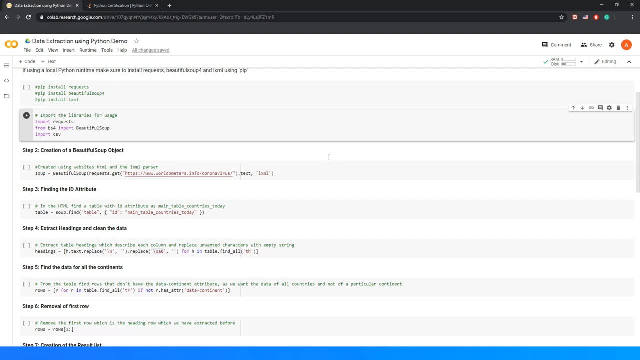 You know, all you're trying to do is making use of the website's HTML, and here is where the LXML parser will come into the picture, And we're trying to create this object where, you know, we're getting all of the source. 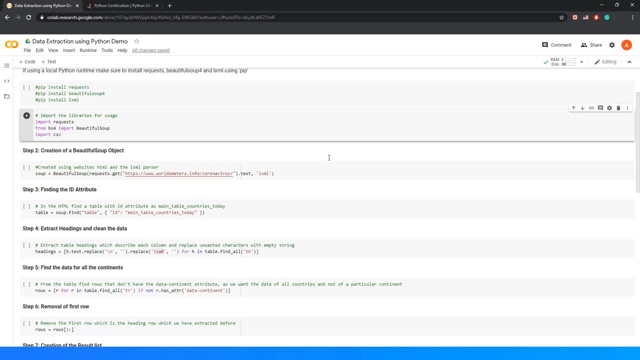 from the website URL as well, So you can see the URL is given on your screen. It's worldometersinfo- slash coronavirus. So this is where all our data is, and all we're trying to use is make use of the get operation in HTML requests. 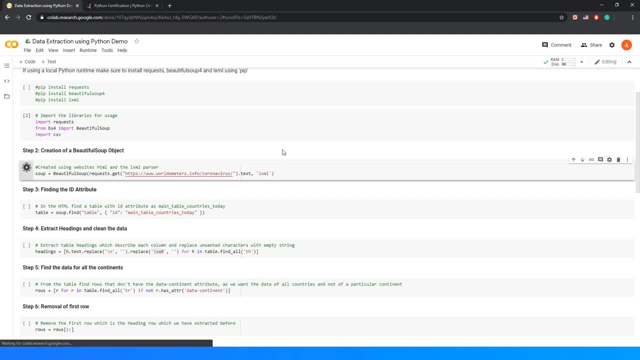 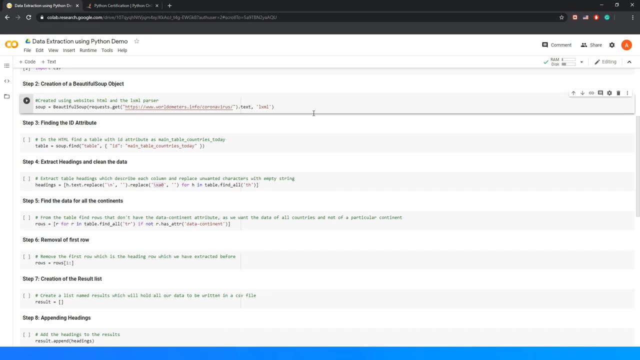 to basically pull all of this data. So by running step two, you've created an object. Step number three is: you know something simple as well. So what we're trying to do here is we're trying to create tables with all of the data. 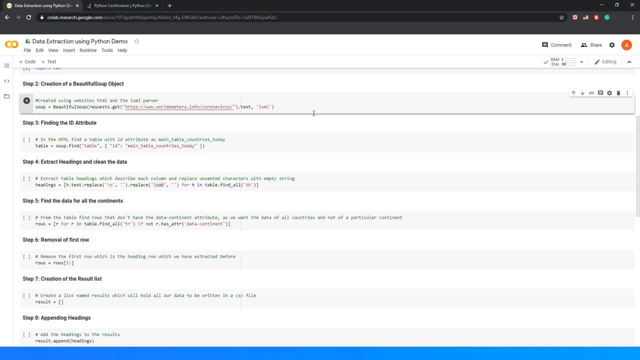 surrounding COVID-19, right. So when we're trying to do this, we need to understand that there are multiple tables which will be available in that worldometers website, So we need to perform some analysis in the backend to find out what table ID is given. 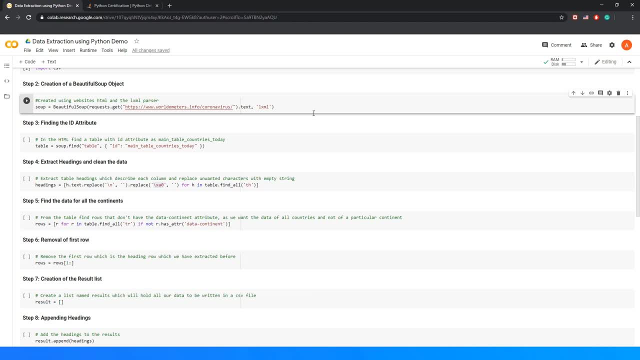 So you know, we can pull all these data from that particular table as well. So here the ID attribute, which I found out to be the table there was given as main table country, And running this will basically create a table. It'll find us the ID attribute. 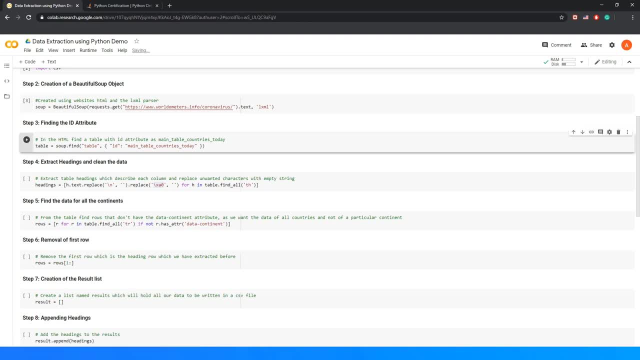 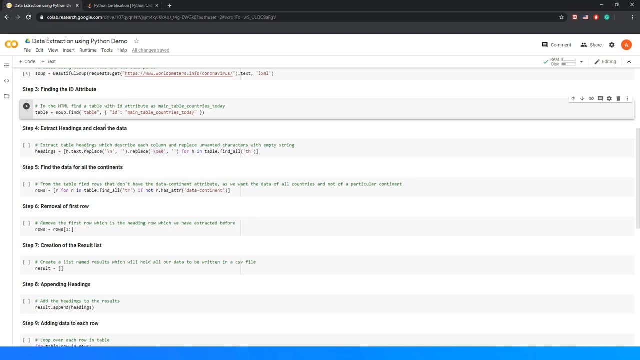 and at the end of the day. so our beautiful soup basically understands that. this is the table, this is the ID where I can pull all the data from. So step number four is basically where we go on to extract the headings that we require for the data chart. 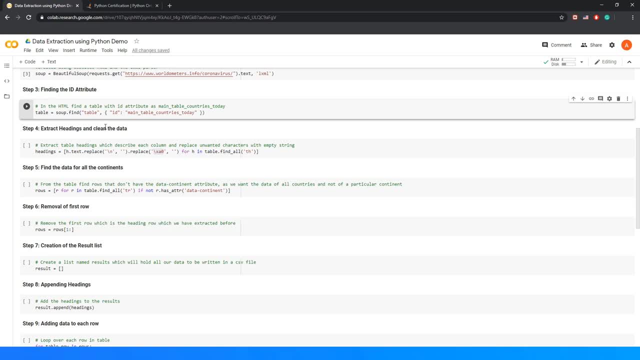 that we're going to use. So, to do all of this, you might be wondering, you know, is the data already clean? where we can, you know, directly grab the data and start using it? Well, the answer is no. 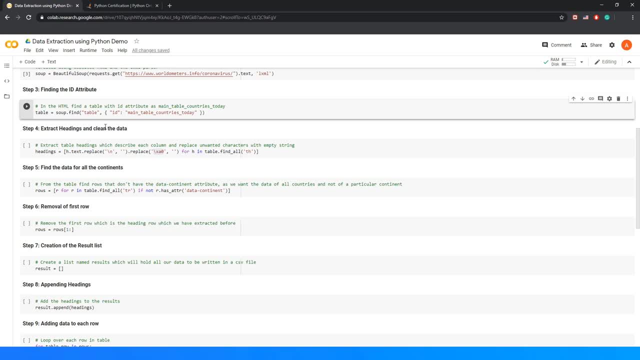 because, with respect to most of the data, most of the cases, the data that we see and use will basically be some sort of you know, it'll have some sort of an anomaly or it'll have some sort of characters where you know we would not want to use. 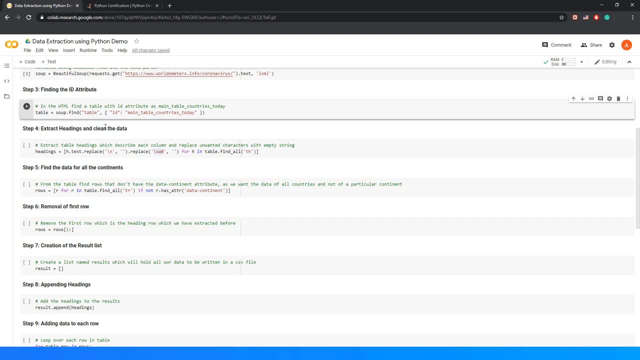 or let's say, it's of no use to us. In that case, what we basically do is, you know, we replace all of these unwanted characters with something else And we make sure that you know we actually go on to keep the data. 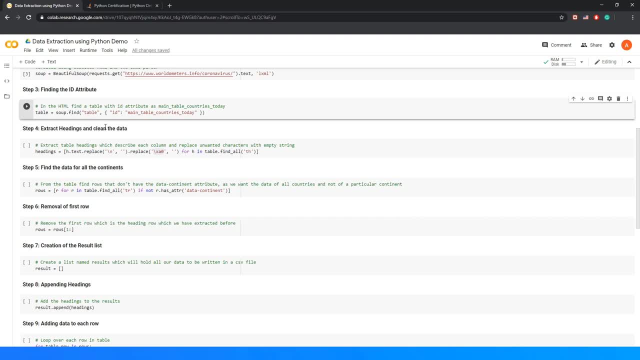 as clean as possible for further use as well. So you can, for example, see: every new line character here is basically replaced, You know, by a blank space when you're working with heading and you're working with a non-breaking space as well. 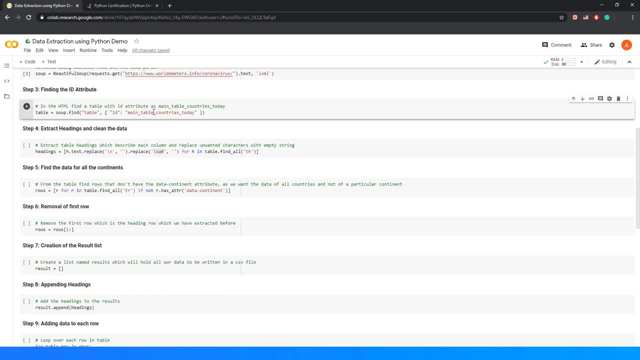 So slash XA0 deals with non-breaking spaces, And again we are replacing those non-breaking spaces with an empty string as well. So all we're trying to do in step number four is clean the data and get all of the headings so that you know. 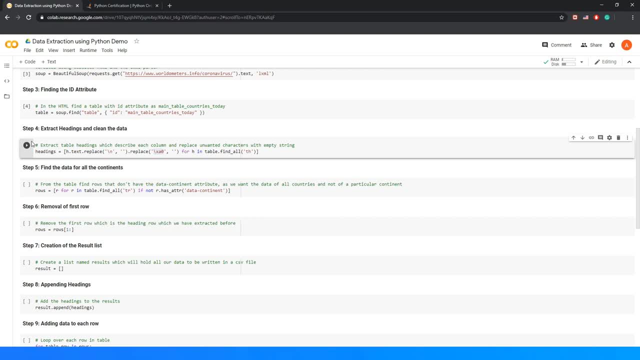 we can have headings for our columns and use it further as well. And after step number four, step number five is to find the data for all the continents across the globe. So, for example, in the data that we have analyzed there is the data: 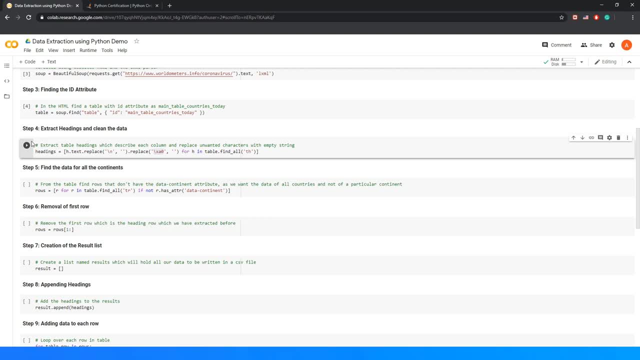 continent aspect where you know data can be pulled for each continent. So in our case, we want the data across the world, right? So we're not looking for data only from, say, Africa, Australia, only from Asia or whatever it is. 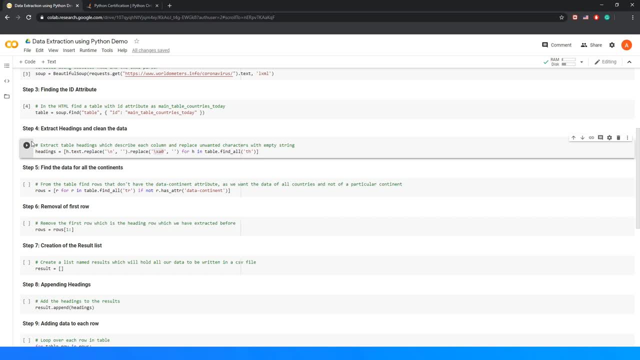 We want the details from across the world. So all we're trying to do is to ensure that we find the table where you know all of the rows which do not have a data continent attribute. So if it does not have a data continent attribute, 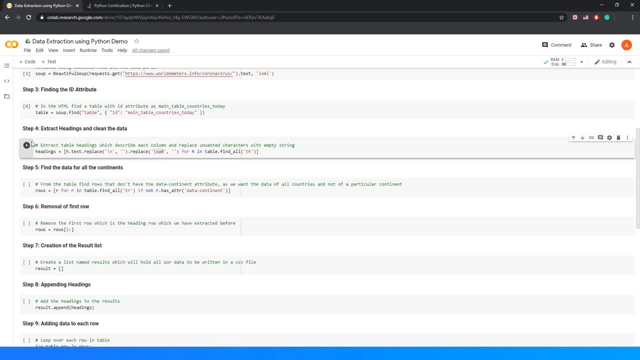 it means that. so we're trying to pick up the data from all the countries and not just any one continent, right? So we want the data from around the world. To do that, we need to recursively go on to check if these particular aspects have. 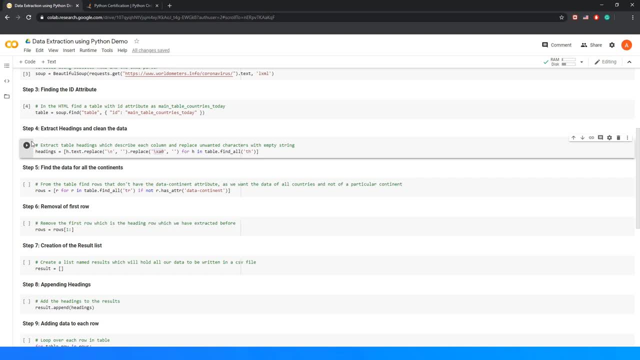 the country's attribute and to find out if these attributes are present or not. If they're not performed, then we're going to pick that, because that indicates you know we're looking at all the countries and not just one single continent as well. 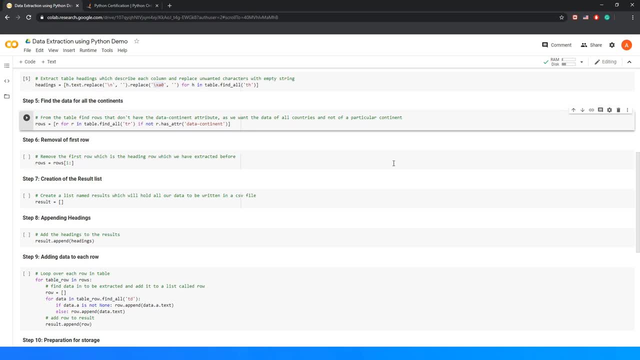 So, basically, after performing analysis and after setting our scope to the data across the world and not just one particular country, we need to remove the first row. So, basically, all we're trying to do is we're removing the first row in the heading. 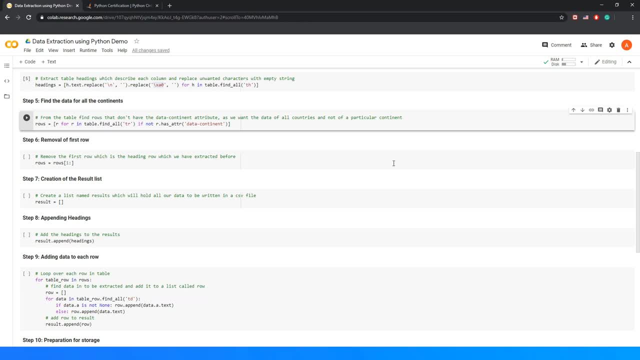 because we already extracted it before, right? So, if you remember, we already pulled out headings in step number four. So basically, performing this operation will remove the first row, since you already have it. to repeat it again Now, coming to step seven. 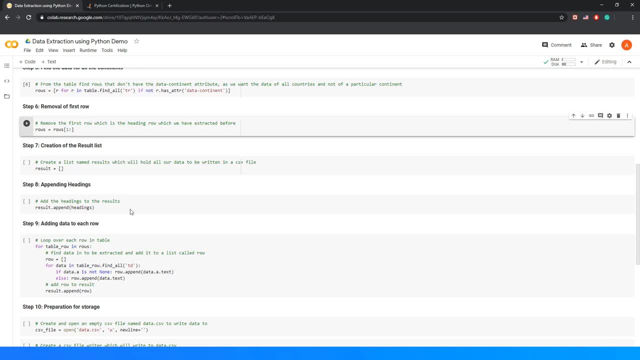 Step seven is basically the creation of the result list. So all we're trying to do here is we're creating a list and we're calling it result, And this list will basically hold all of the data temporarily until it can be written into a CSV file. 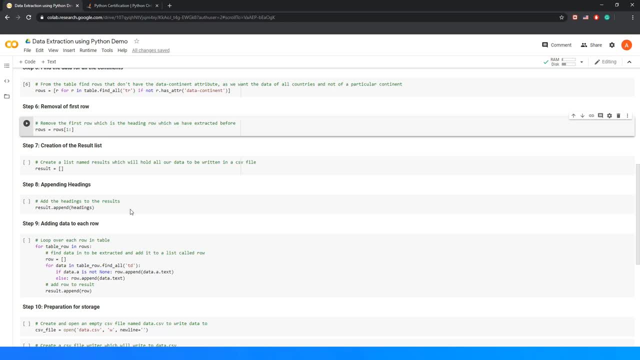 which will be our final output. So let me repeat, We're going to create a list, called as a result, and this result will be a temporary point of storage for all of our data, which will later, you know, be written in a CSV file. 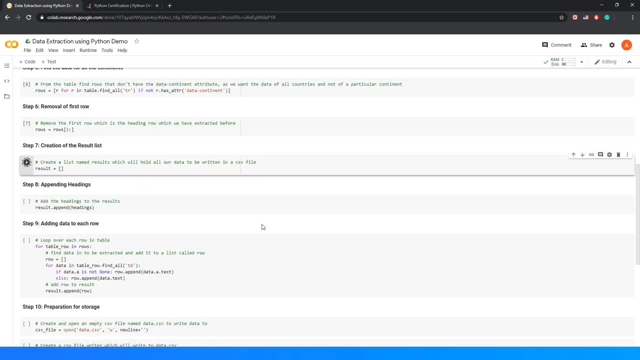 and this CSV file will be our output. So basically, running step number seven will create the list. So basically, at the end of the day, we need to append all of these headings. We need to add all of these headings to the list, right? 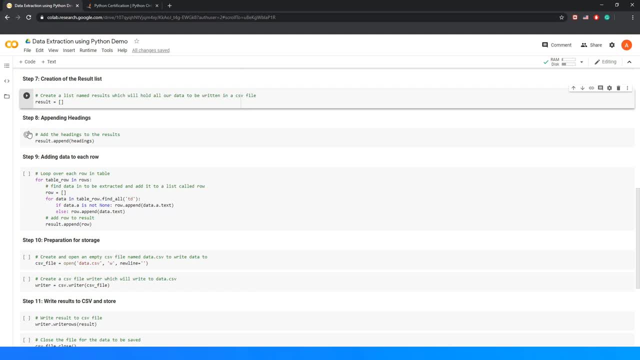 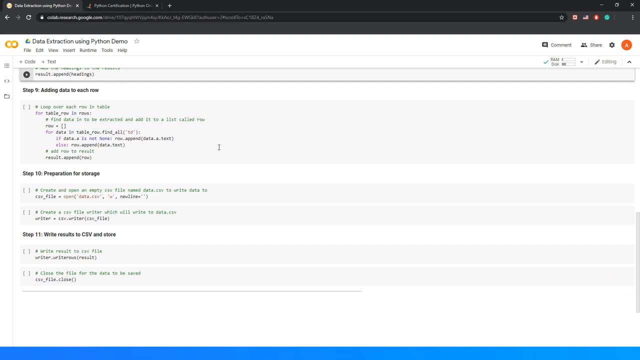 So result dot- append of headings will do just that. It will make sure to add all of the heading to the results that we actually want. And step number nine until step number eight. we have, you know, cleaned the data. We have pulled all the data. 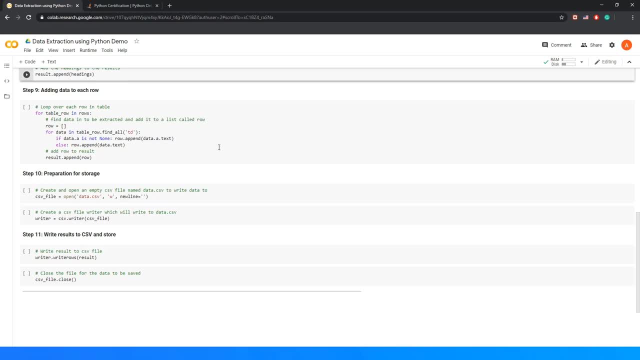 that's required. We have created headings and you know we have basically removed all the unwanted spaces. We have created a result list and we have added the headings there. Now, step number nine deals with adding all the data with respect to each rows. 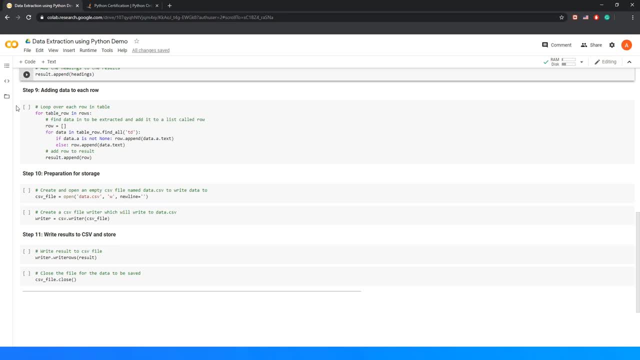 and each columns as well. So until now, we already picked up the headings with respect to step number nine. So, step number nine, we are going to basically find all the data that needs to be extracted, to find all the data, to scrape all the data. 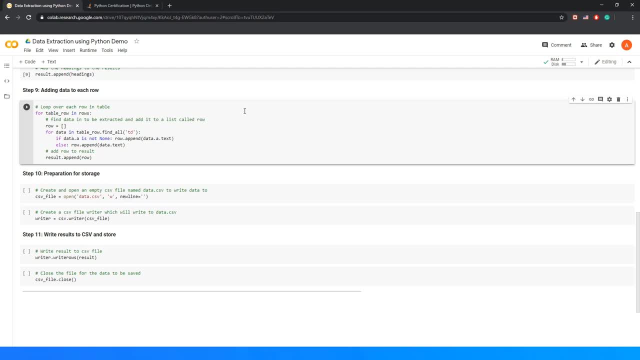 and we're going to add it to a list called as row. After we're adding it to a list called row, we're going to check if it's present already. If not present, we're going to keep adding it And after that. 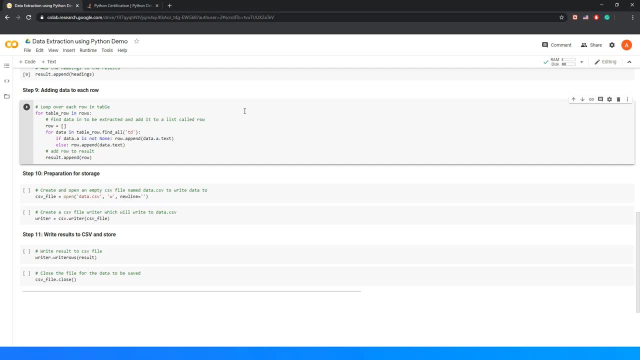 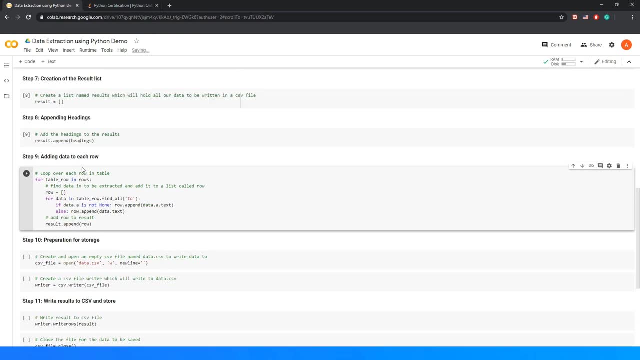 we're going to have to add all the data that we found in the row list into the result list, right? So basically, the row list will have all the data that we have pulled through, all the different rows in the data, So it will not have headings. 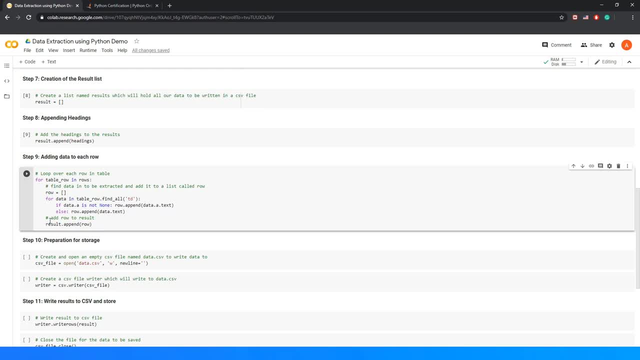 at this point of time, To make sure that the data is collaborating with the headings, which is basically present in our result list, we actually append the rows to the results as well. So performing step number nine will add all the data to each particular row. 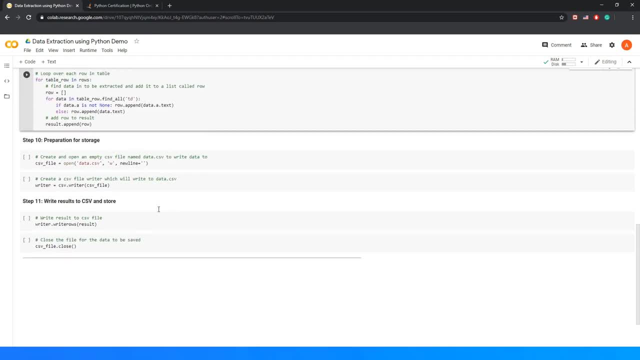 and eventually append all of this to our result list. And then step number 10 is the most simple step, probably because here is where we are preparing for storage. So whenever you create any file in Python, basically be it CSV file or anything, we need to create a file. 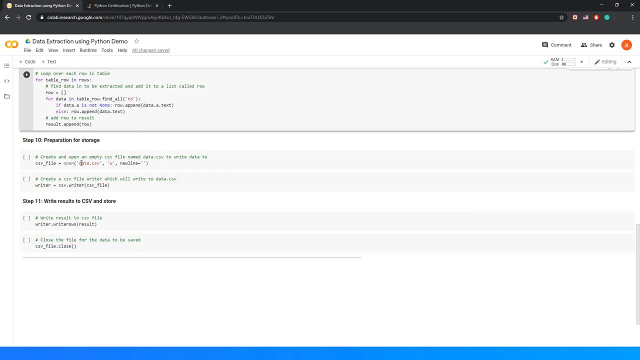 and we need to open it as well. So basically, using the open command, we're creating a file called as datacsv and we are opening it in the write mode and we're starting it with a blank line as well. So when you go on, 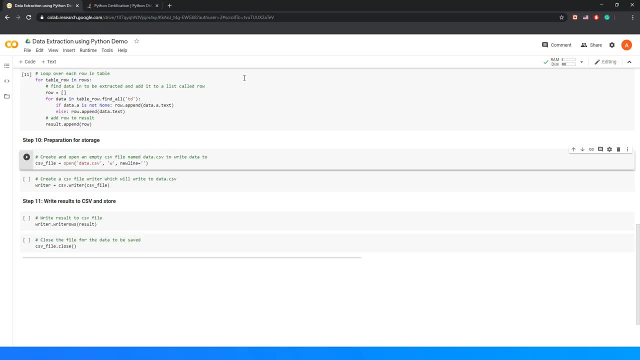 to run this particular command in step number 10, it will create an empty file. It will create a file called as datacsv. It will open that file for further working because we need to write the data right, So the file writer needs to have access. 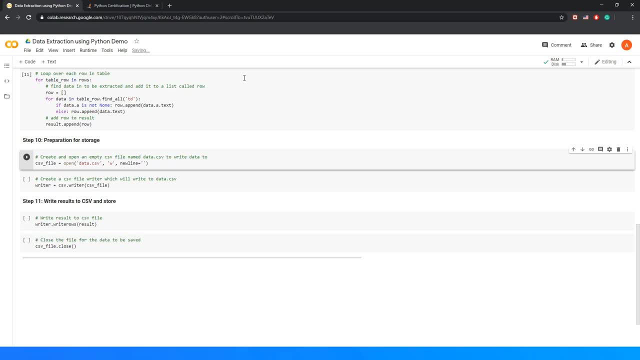 to all these files that it can write to. So that is why we open it. you know, prior to writing. And again, the second part of step 10 is to actually write these files- that we actually obtained it into this file called as CSV file. 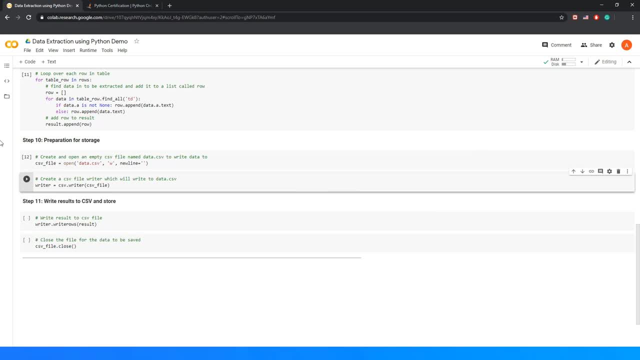 And then we can actually push all of these results. You know, step number 10 was basically preparing it for storage, creating it, opening it and make sure that there is a file writer which can write. Step number 11 is where we actually write. 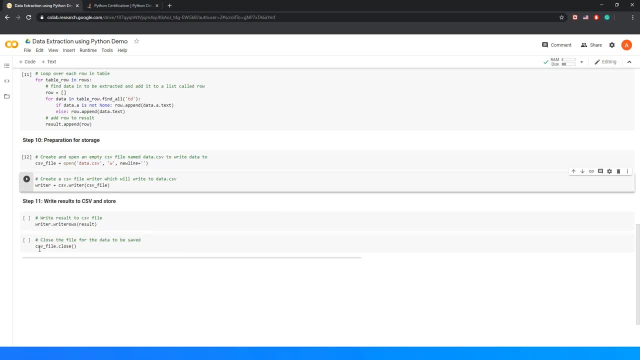 the result into the CSV file. So writerwriteRows of result will write the actual results to our CSV file. This will be pushing, you know, all of the data that we have from our result list into the CSV file And at the end of it. 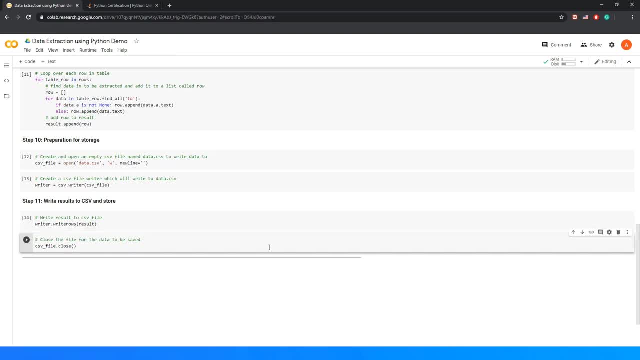 it is always a good practice to you know, close the file, basically, which will make sure that the data is saved. So you might be wondering now: okay, step number 11 is done. We've written everything to the CSV file and it is stored. 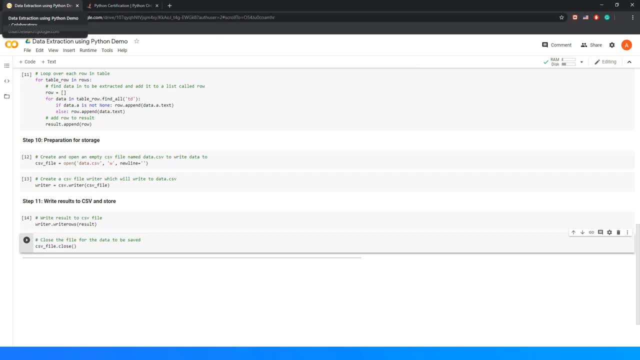 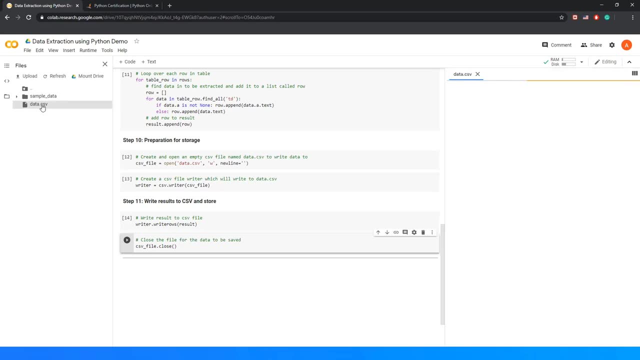 But where is the file? Well, in your case you will have the file present in the Python interpreters folders. In our case, it will be created basically in the Google's Google Ecosystems files. And let me double click on the datacsv. 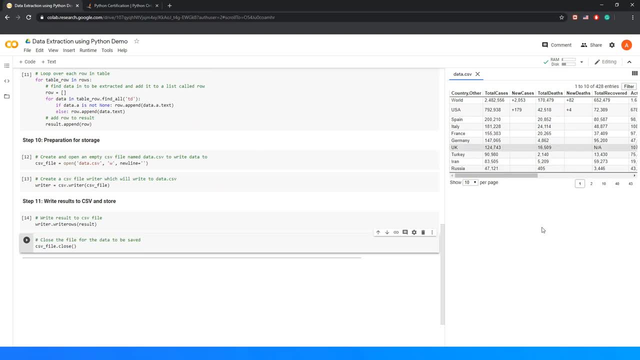 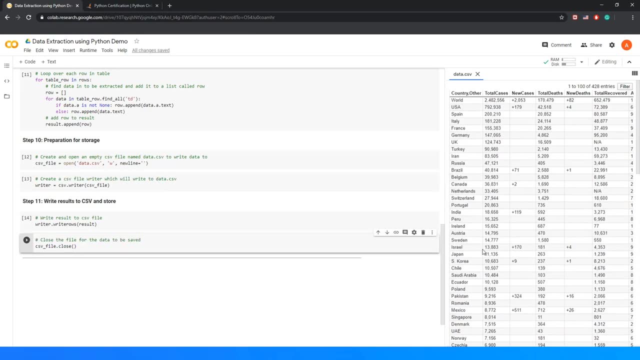 that we just created here And, as you can see on the right hand side of your screen, you can, you know, choose to pick up how many ever details that you have to show on your screen as well. So here as well, you know. 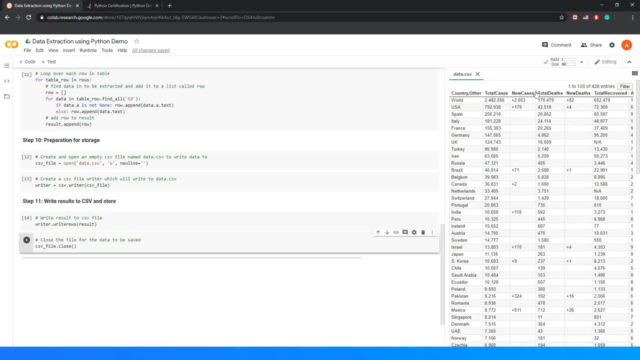 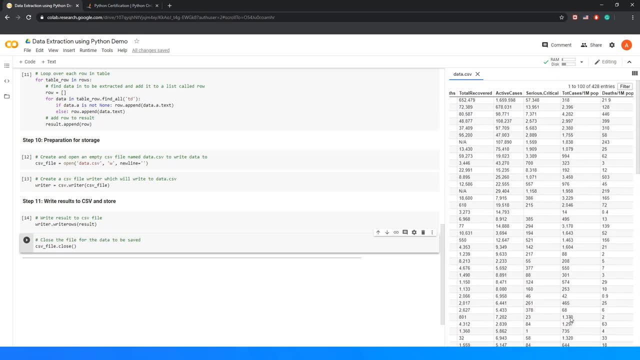 all the countries, all the total cases, the new cases from yesterday, the total number of deaths in that country, new deaths, total recovered and much more So. this detail, you know, we've picked up from the Worldometer side. What are the active cases? 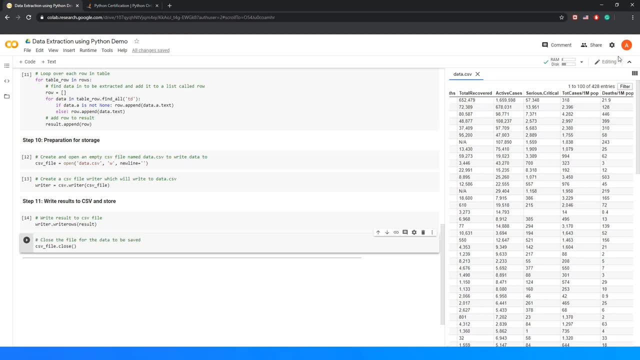 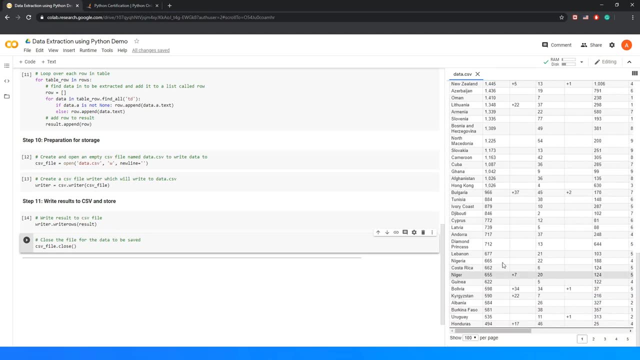 How many of these active cases where people are serious, What are the total cases for 1 million of population? deaths per 1 million population and much more So. Worldometer- this is a comprehensive website, and this at the end of the day. 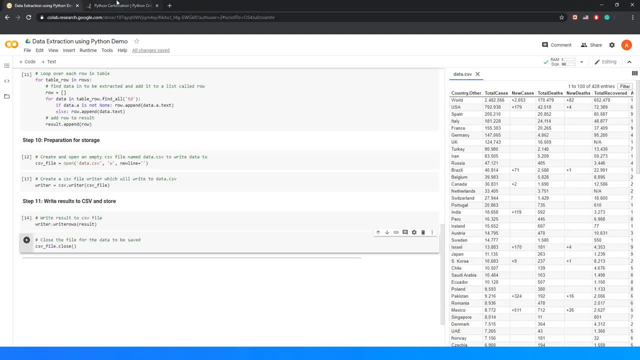 you know, this will create a very nice data set, and this data set, at the end of the day, can be used to perform analysis Again. to find out how that is done, make sure to check out our machine learning video, which is basically performed. 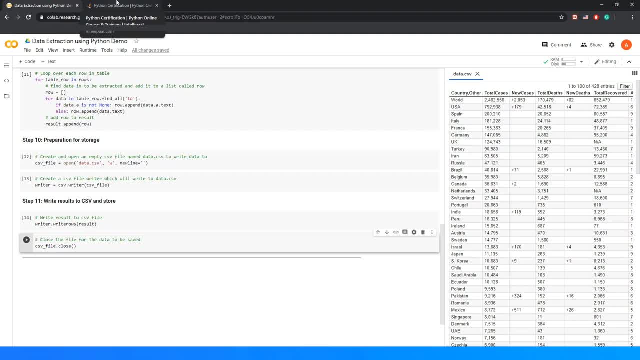 using the data set similar to this as well. So this creation of data set not just in the case of COVID-19, it can be anything across the world. Once you have structured data and once you've created structured files like this, you can understand that. 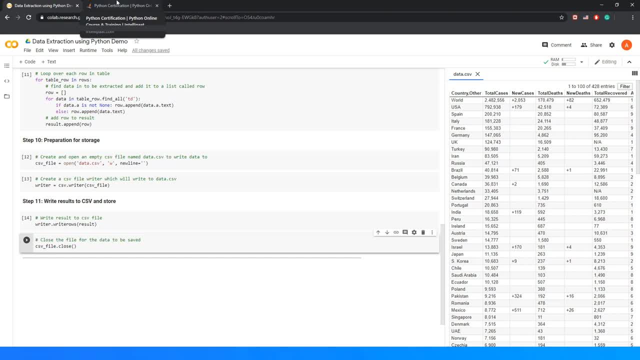 you know, you can use this and make full use out of it down the ladder, Down the ladder. it's basically performing analysis. It can be, you know, working with deep learning, working with machine learning, whatever it is. Step one is very much essential. 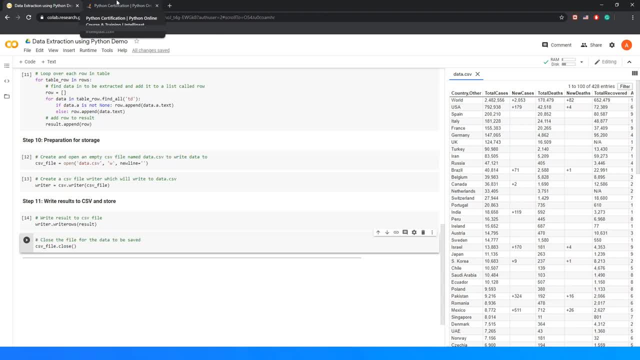 in all of these fields of processes, and step one is creation of data, And you know we have created a structured pipeline to access our data as well, And this, again, in my opinion, is one of the most important use cases, or 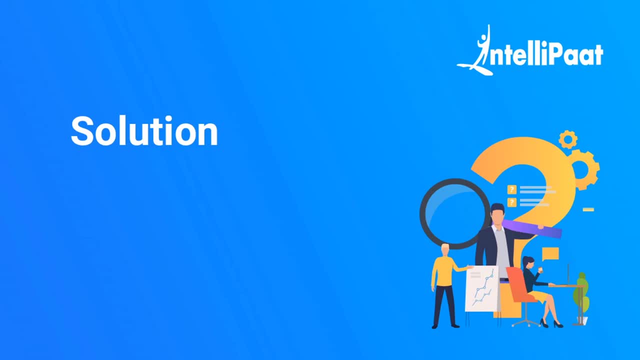 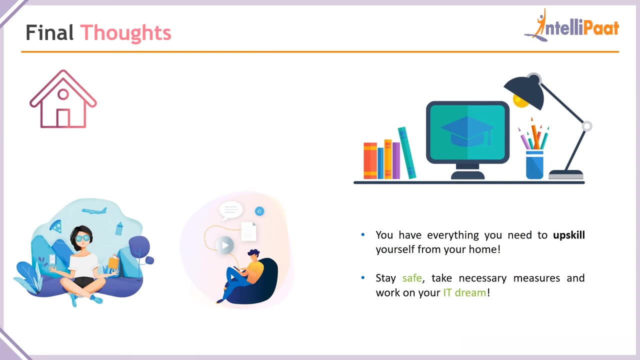 you know uses of data extraction when you're working with Python as well. That brings us to my final thoughts on this particular presentation. Well, guys, at this moment of time, guys, you need to know something. It's that: data extraction. 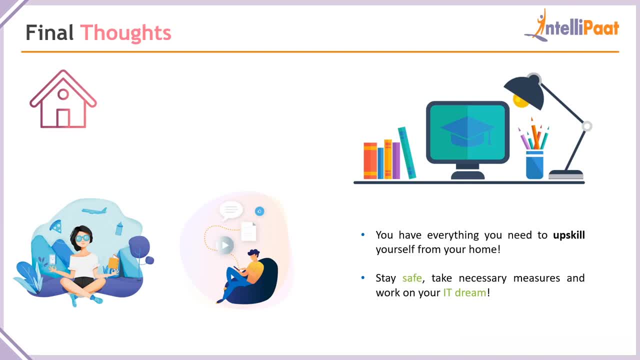 using Python is very powerful is the number one point. The second point is that you know, even in so, even in quarantine, even being safe, right now you have everything at your home to pretty much upscale yourself If you have a valid. 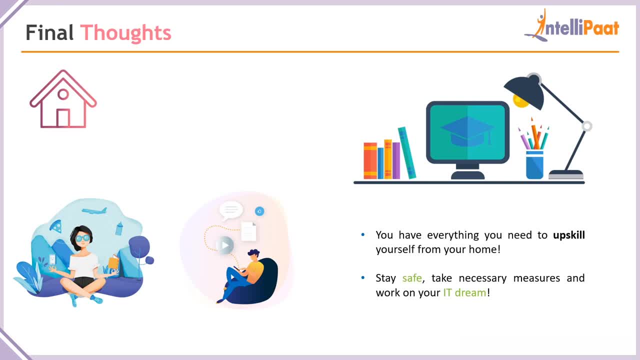 internet communication. if you have your phone or if you have a laptop computer, you can basically use it to do everything you can. So stay safe, take every necessary measure that you need to stay safe and, basically, you know, don't let this hinder. 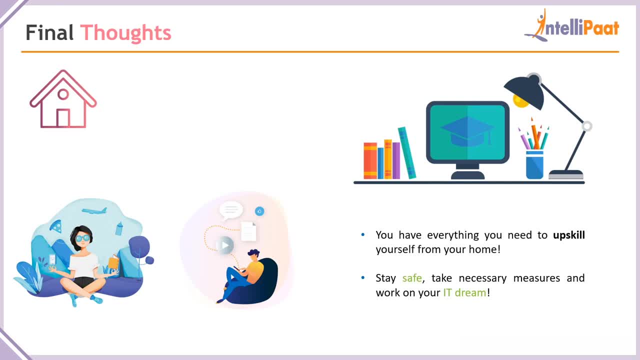 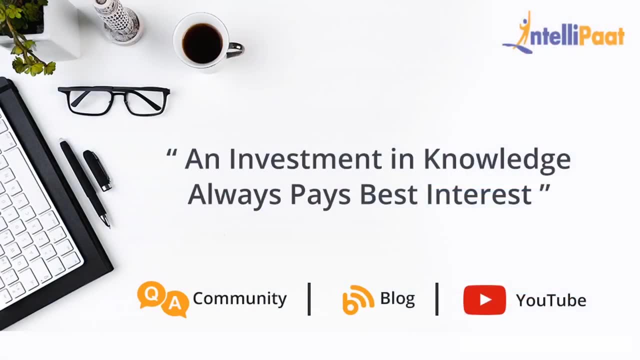 your IT dream, or to help you, you know, get on to your dream IT path as well. So make full use of this to launch your IT career as well. So for further learning, what can you do At this moment of time? 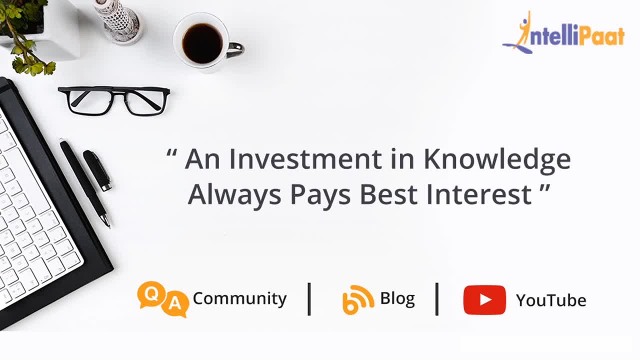 I'd like to tell this quote saying: an investment in knowledge always pays the best interest. So this is a quote by Benjamin Franklin and it's an amazing quote. So you know, when you read it more and more it gets wilder. 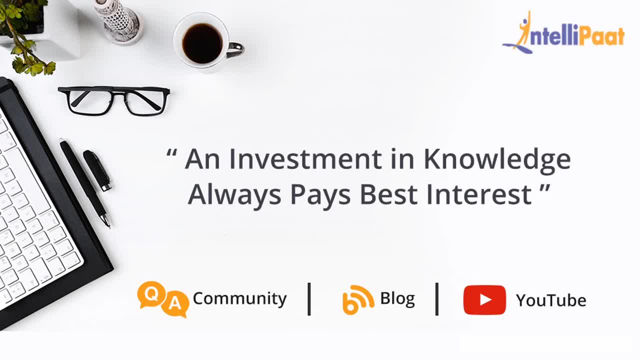 you learn anything comprehensively. Make sure you can check out our YouTube channel. there We have a plethora of content that we put up every single day. So you know, make sure you subscribe, Make sure you hit that bell icon so that you're always. 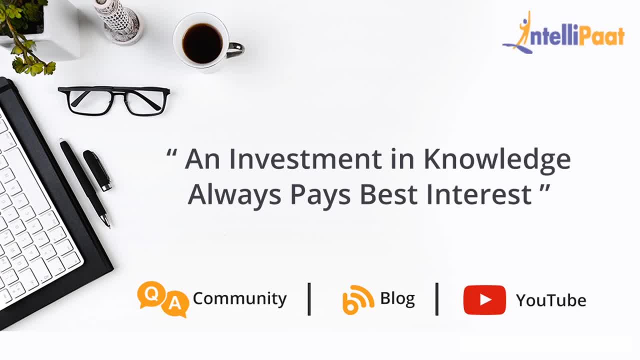 notified whenever we put a video. If you're more of a blog reading person, we have Intellipaat blogs. Make sure to Google it and you know you can get access to a wide variety of content that our blog writers write for you as well. 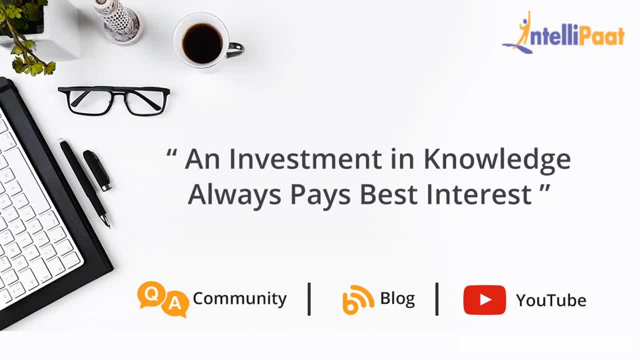 And we have the Intellipaat community where you know we have a friendly community like Intellipaat community as well. So basically you can ask any basic question all the way to the most advanced- you know- programming question where you might need. 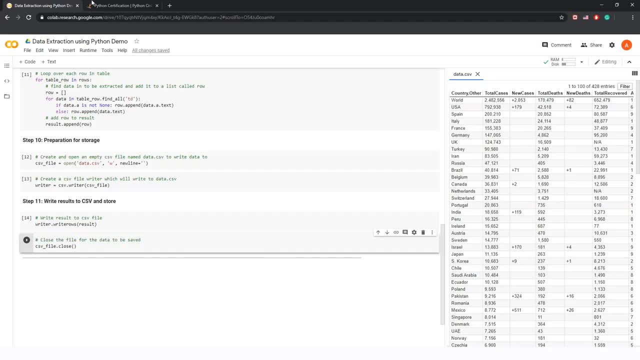 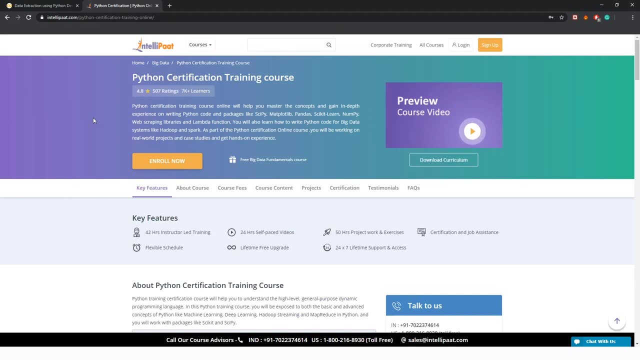 help with something, And our community will be more than happy to help you there as well. So, on that note, as I promised, let me show you the fastest way you can learn Python. I present to you Intellipaat's Python certification. 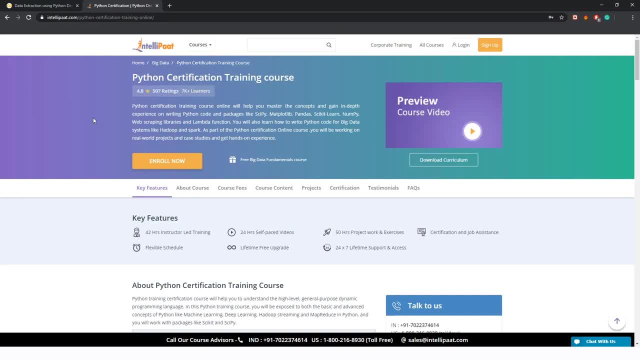 training course. This is one of the very well-reviewed course and all of our learners love this. So we have over 7,000 learners, who basically 10,000 learners for this program. You know it contains a lot which will help you. 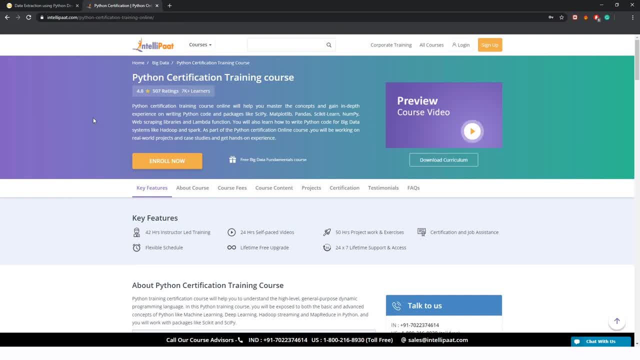 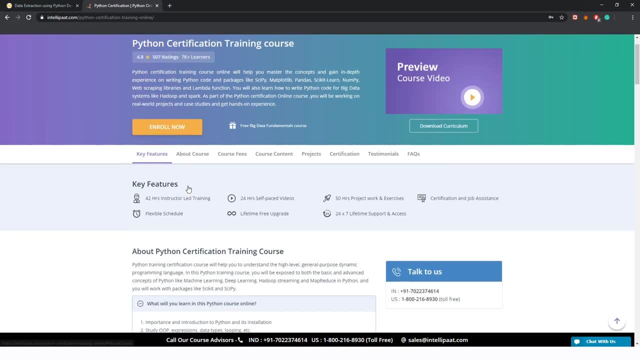 get started from the fundamentals of Python right till you get good proficiency in it as well. Everything from SciPy, Matplotlib, Panda, Scikit-learn, NumPy, web scraping library, Lambda functions- everything will be covered in detail in this course. 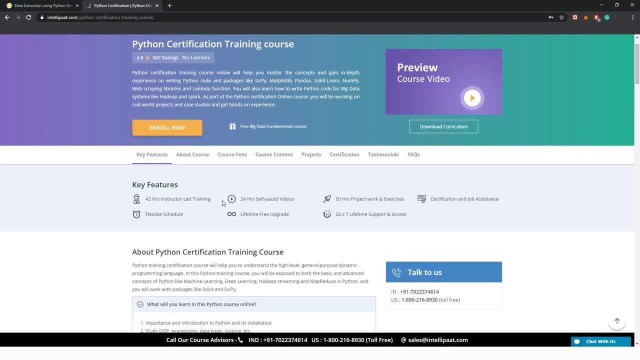 So the key features is that we'll be providing you 42 hours of instructor-led live training, 24 hours of self-paced videos and over 50 hours of project work and exercises. We believe that you need more project work. you need more hands-on exercises. 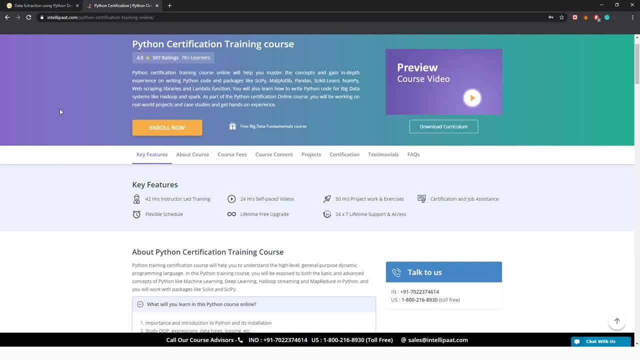 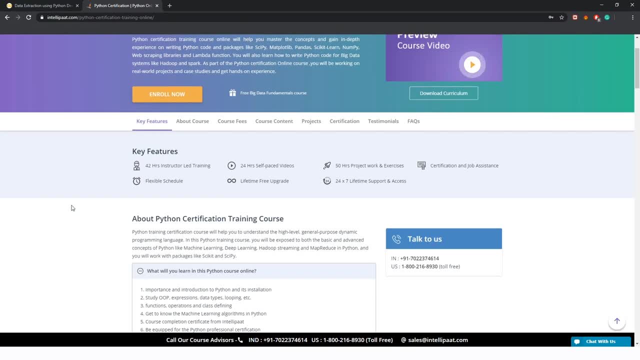 than theoretical concepts and of course, to stand by that, we do provide a lot of industry-level project works as well, And of course, at the end of it, after you finish the program, you will get a course certificate and job assistance as well And flexible scheduling. 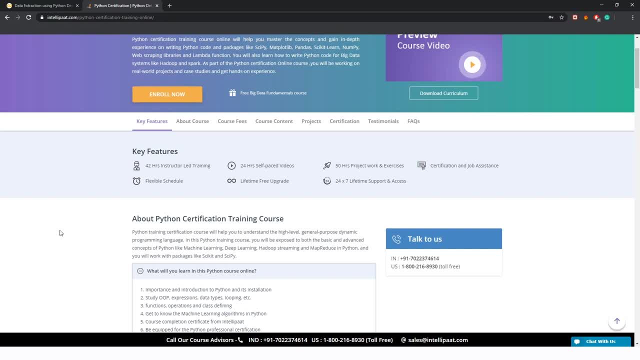 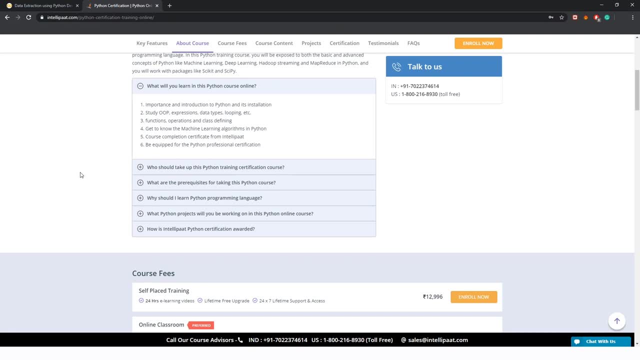 lifetime free access. lifetime free upgrade. lifetime 24-7 support for your courses are something we stand by as well. So you can check out the about section, where you have all the details about the Python program as well. You know what should you learn? 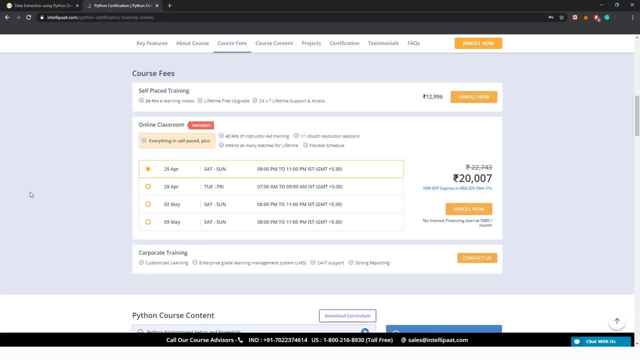 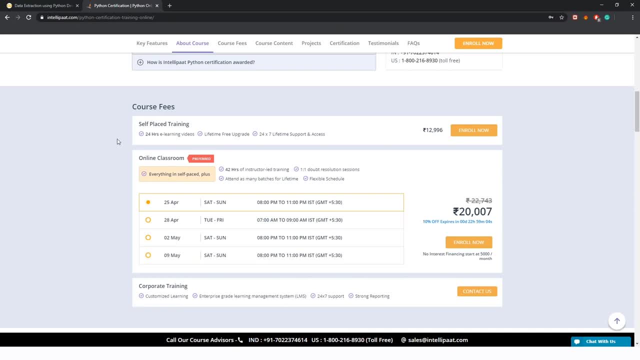 what are the prerequisites? why should I learn Python and much more, And these are some of the batch details that you can check on your screen as well. Again, make sure you give us a call on the numbers you see on your screen to check out. 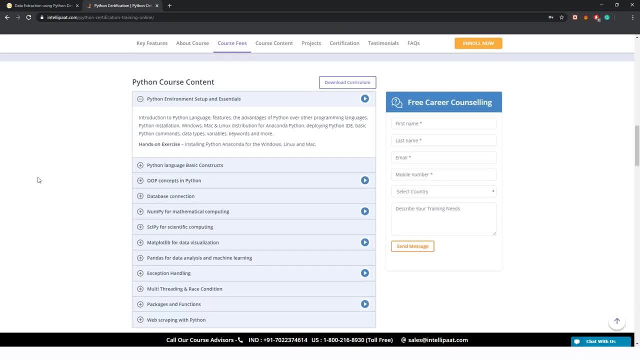 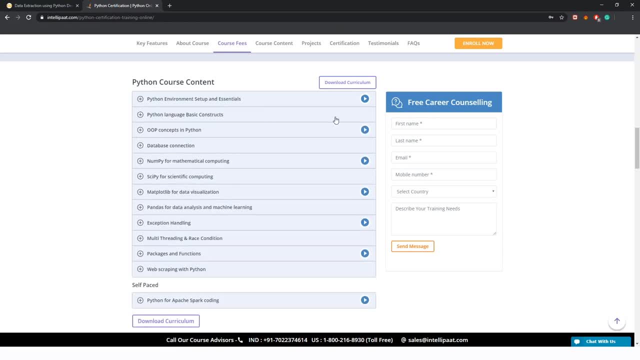 when there is the next batch and you know, to see if you can enroll into that batch quickly as well. Coming to the actual course content, you know you can download the entire curriculum basically by clicking on this link here, and it will allow you to do all the. 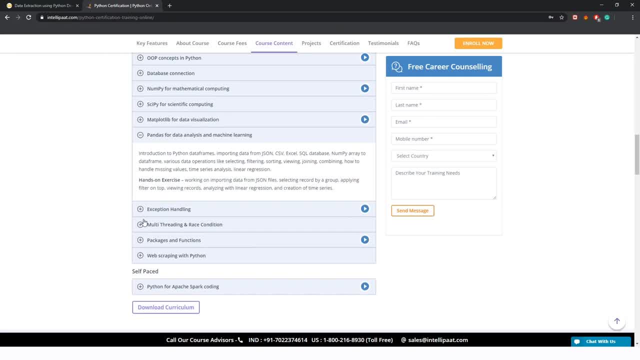 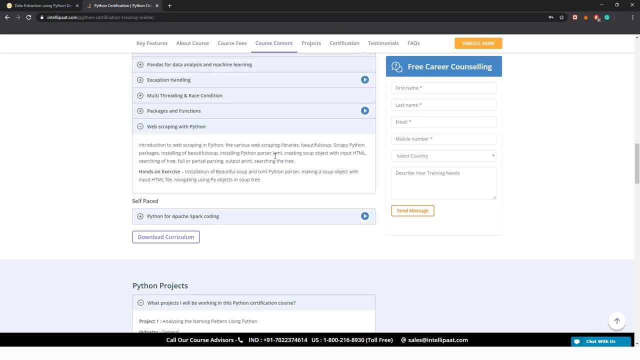 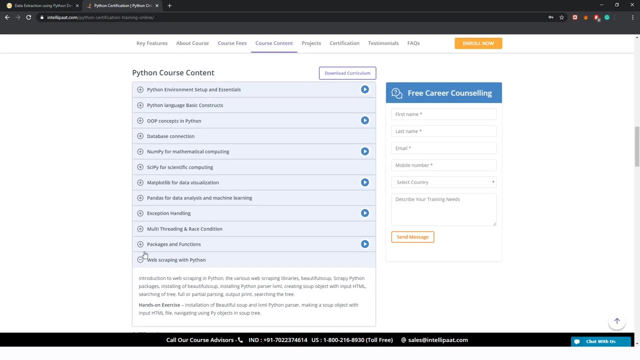 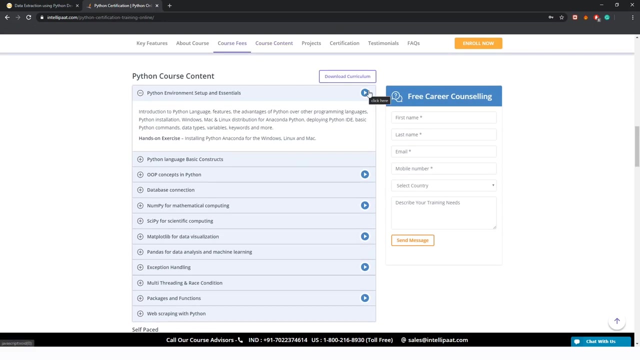 building stuff. so all the skills, everything you need to be able to get that free from Python, is in that video as well. You know, again, you can take a look at some of these and definitely you can learn anything that you want from Python on this. uh, uh, play button here as well. uh, you know, you can get access to the free video of that. 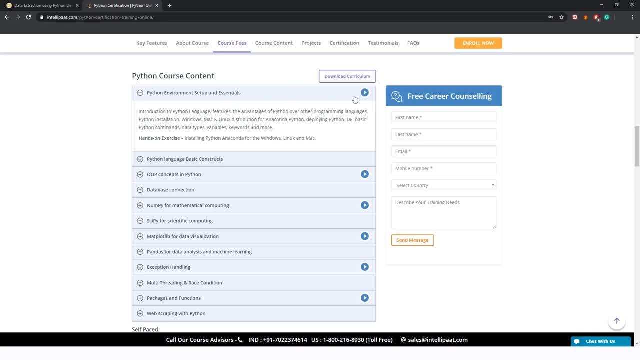 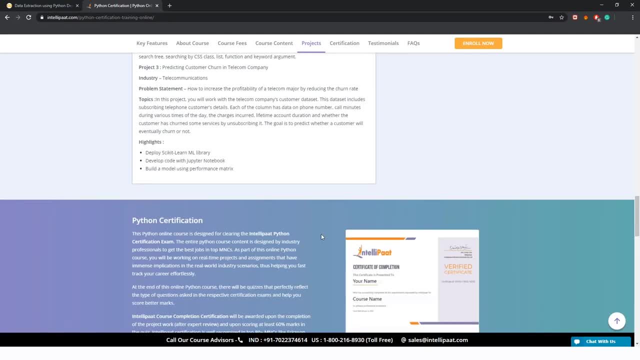 particular module where you can check out a free demo to see, uh you know, if this course is right for you there as well. so, again coming to the projects aspect of it, we have multiple projects, as uh discussed. uh, you know, we have three industry level projects from variety of industries there's. 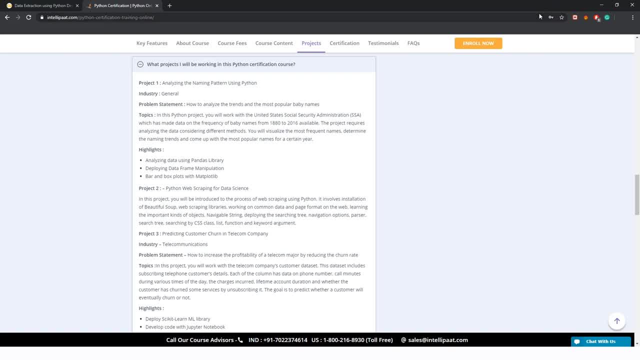 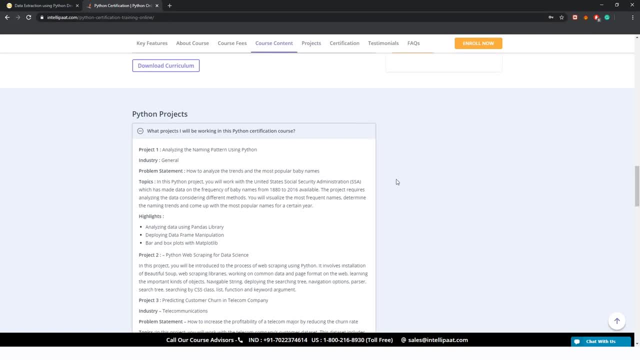 a general industry. there's a telecommunication industry project and much more. we give you problem statements, we give you the topic and we give you the highlights as well, to ensure that there is good transparency here, ensure that you can actually learn. so, basically, to ensure that you. 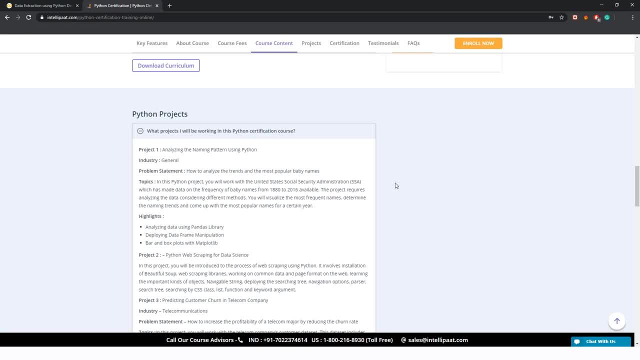 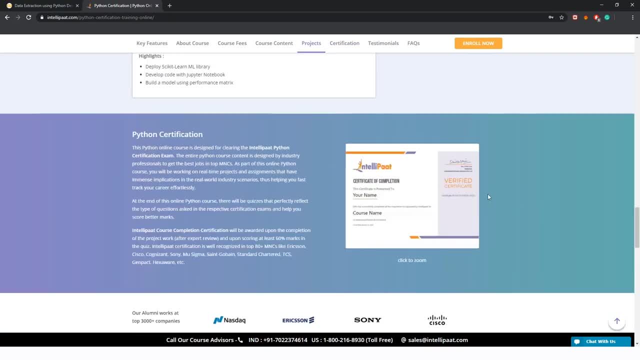 know you implement everything that you learn in this program as well. so, again, there are multiple projects. you work with certifications, we have our testimonials- uh, with respect to all of our learners as well- and at the end of the course you will be given a certificate of completion, which 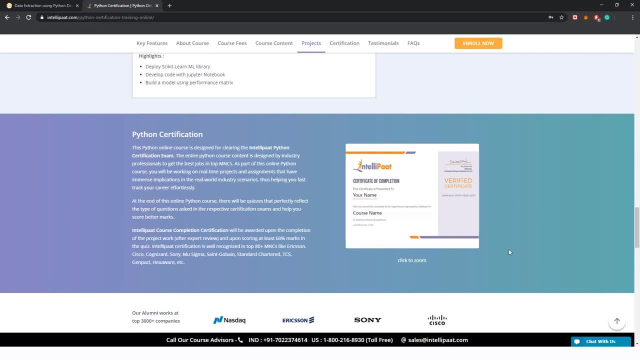 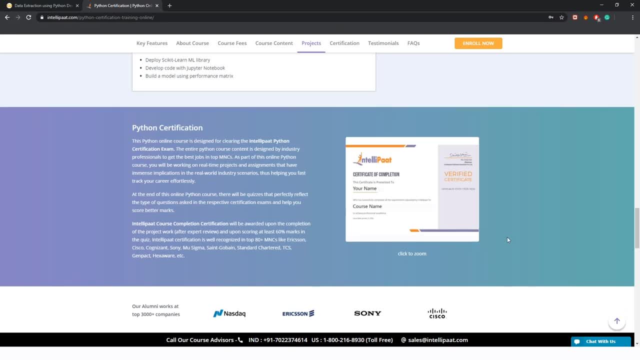 looks just like this. this is very well, uh, regarded and recognized in a lot of mncs. you know everyone from ericsson, standard, charter, tcs, cognizant sony, new sigma, hexaware, genpak and much more. and, of course, all of our alumni work at the top 3000 companies. it might be nasdaq, ericsson sony. 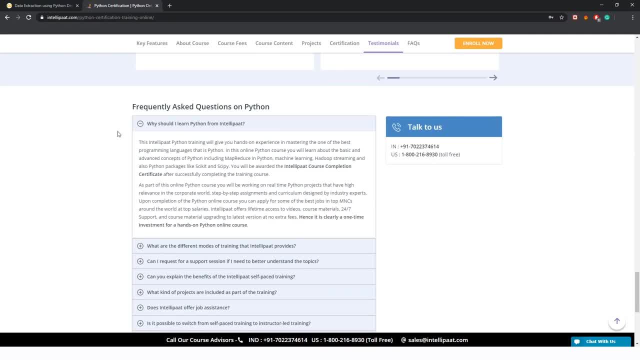 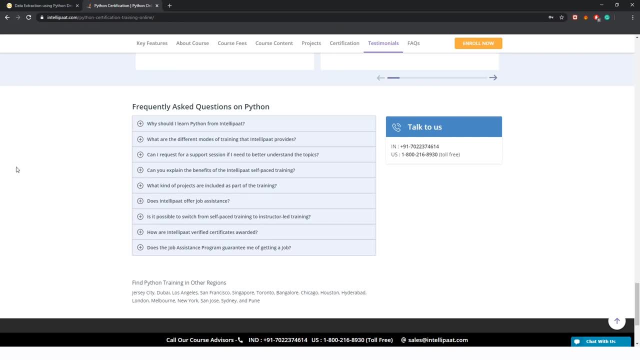 cisco, just as i mentioned, and many others as well, and at the end of it, we know you might have more questions about this, so we've put in an entire faq section which will help you, uh, get better clarity of the course as well, and, uh, we understand that you know you might have more questions apart from.